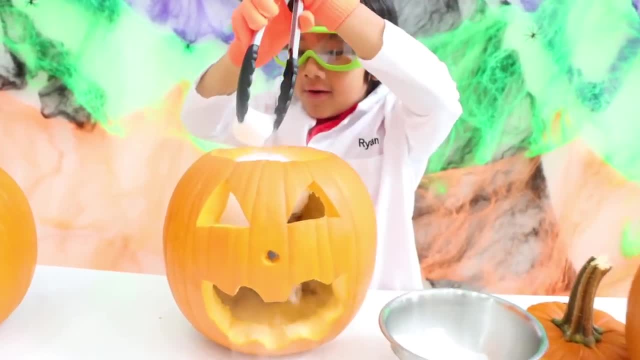 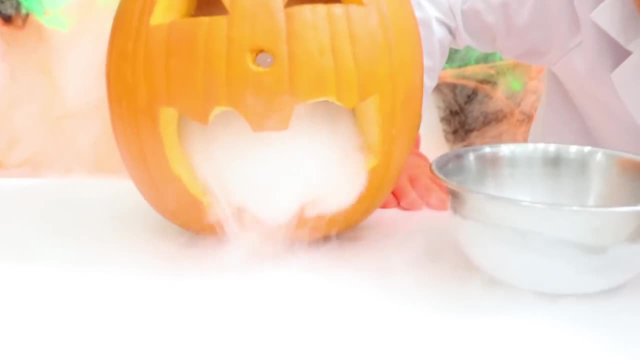 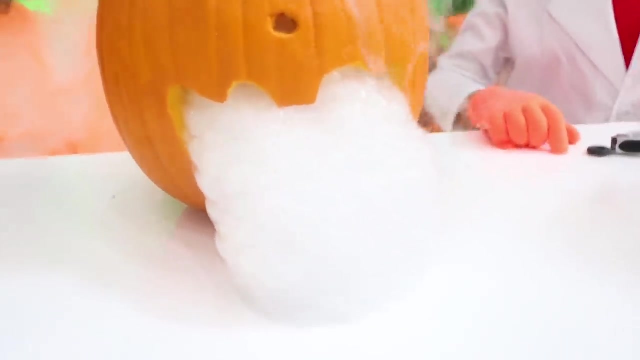 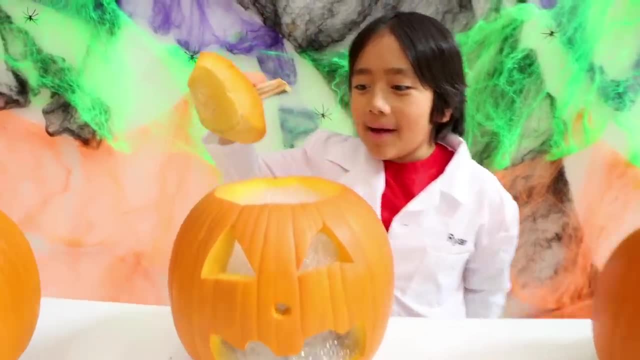 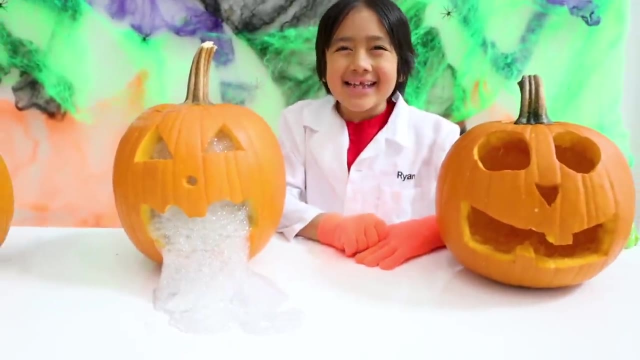 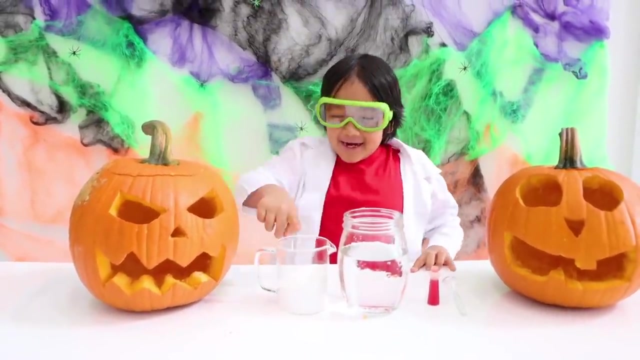 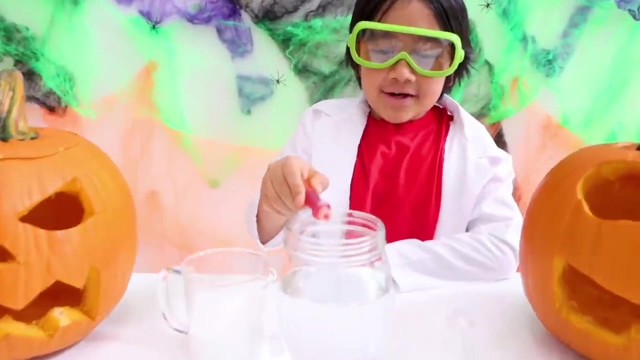 Out of the eyes. Whoa, there's so many bubbles. Whoa, that's so cool. Okay, guys, On to the next experiment, Next pumpkin experiment, the classic Baking soda and vinegar. So first I'm going to add some food coloring into the vinegar. 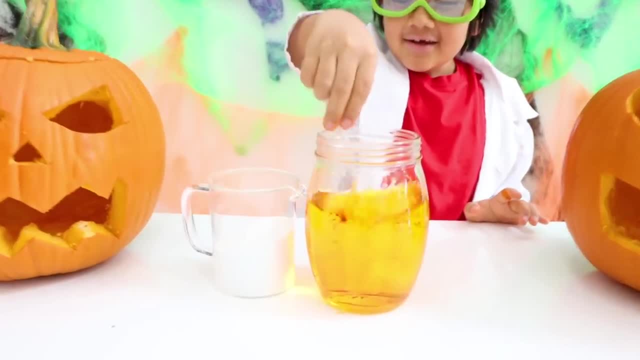 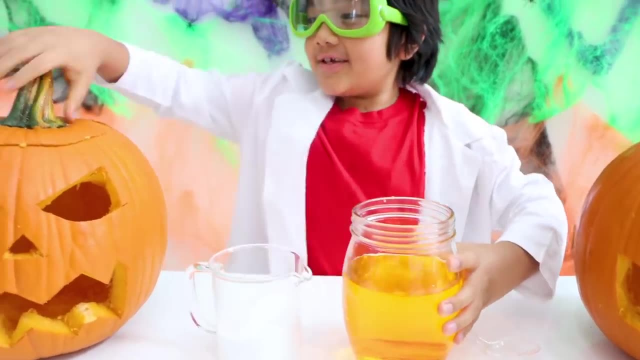 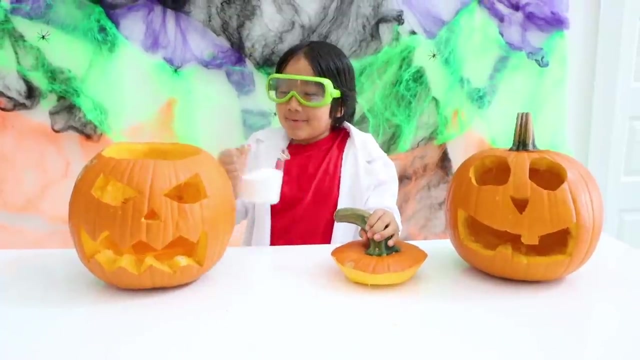 Maybe that much Agitate, agitate. Now it's orange. Next I'm going to put it into my par with jack-o'-lantern. Okay there, Next, put in the baking soda and then close it right away. Whoa. 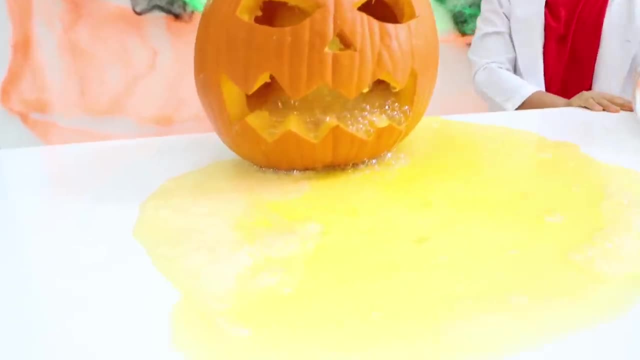 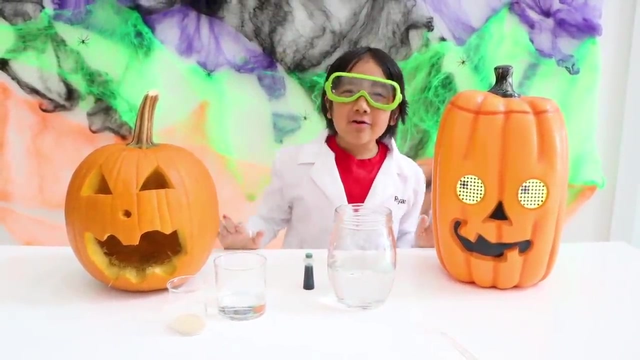 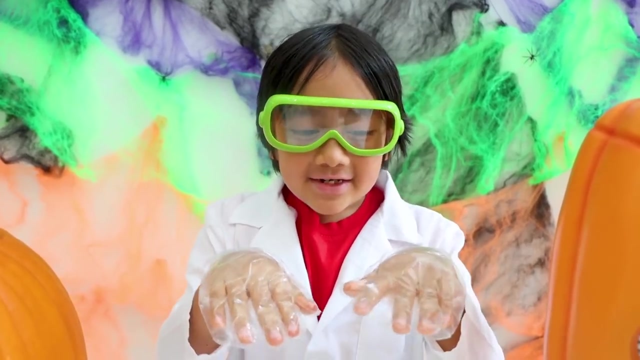 My right away was not that fast. Now we're doing the last experiment, But it's my favorite elephant toothpaste, So first you need hydrogen peroxide. Be careful, It's not good for your skin, So wear gloves, like me. 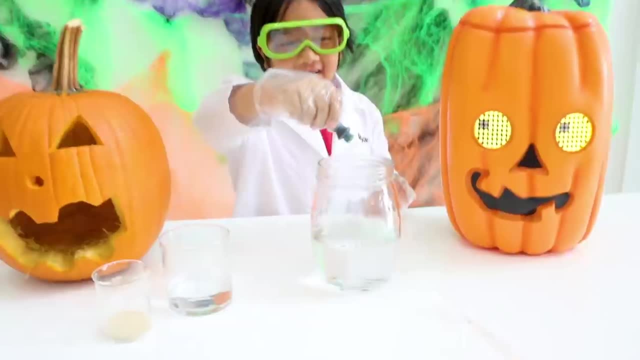 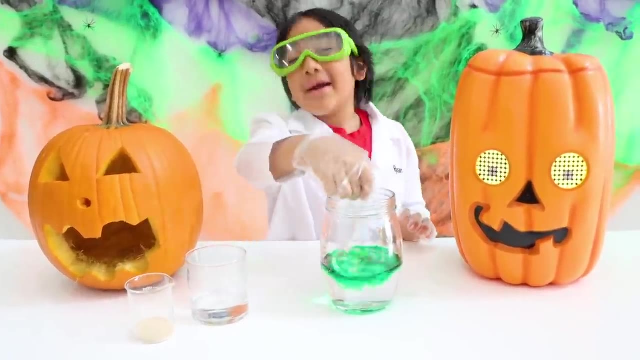 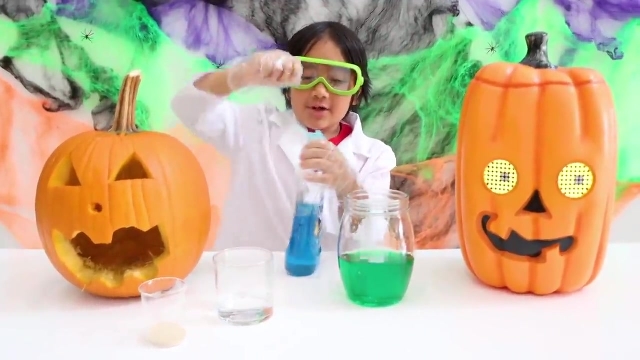 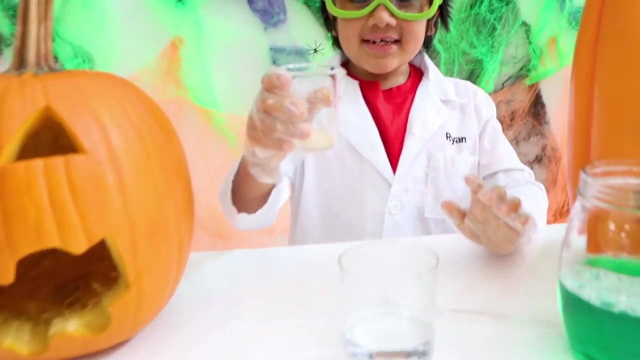 Next, I'm going to add a few drops into the hydrogen peroxide. You can find hydrogen peroxide at the beauty store. Parents know that. Next, I'm going to add a few squirts of Dawn soap- One, two, three. Next, find some dry yeast and add it to warm water. 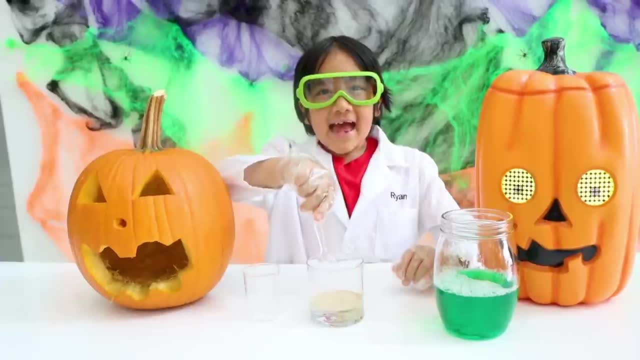 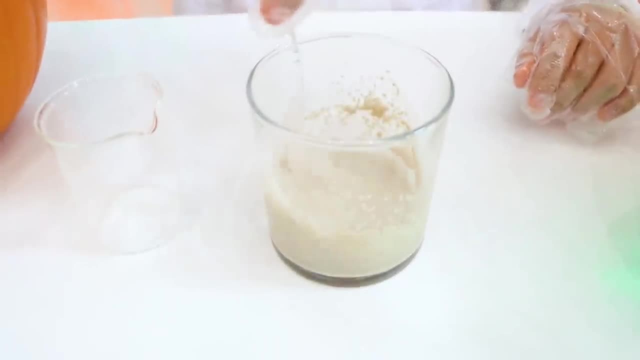 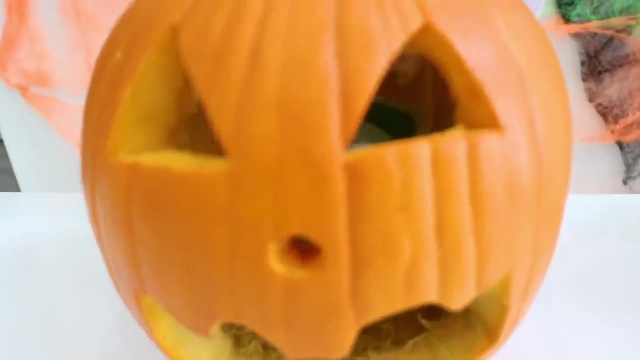 Then we agitate: Boom, boom, boom, boom, boom. Next, add your hydrogen peroxide into the Jack-o'-lantern. Okay, okay. Now here's the fun part: Add the yeast and then close it. Whoa. 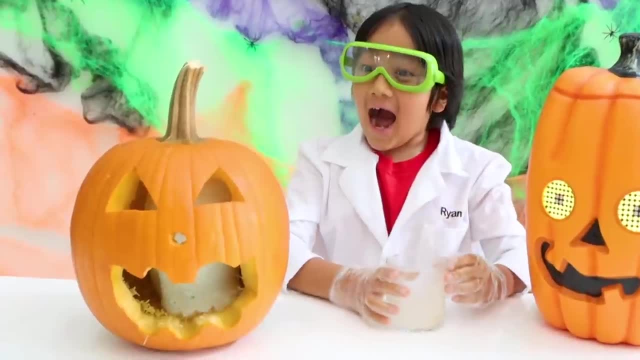 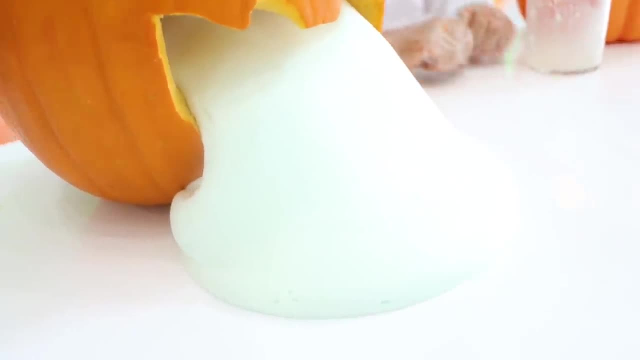 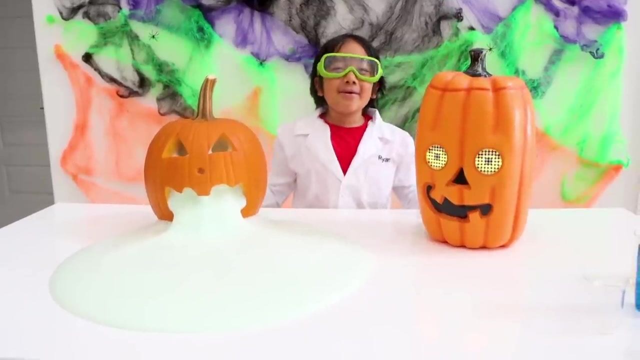 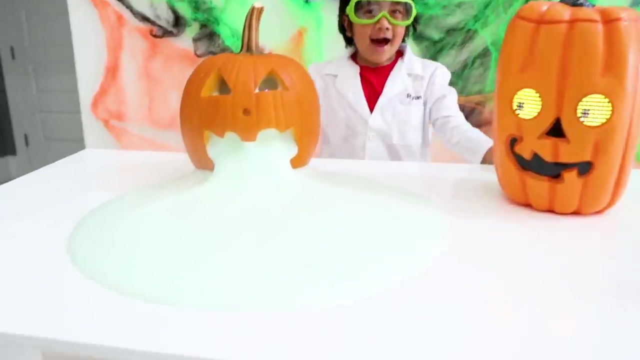 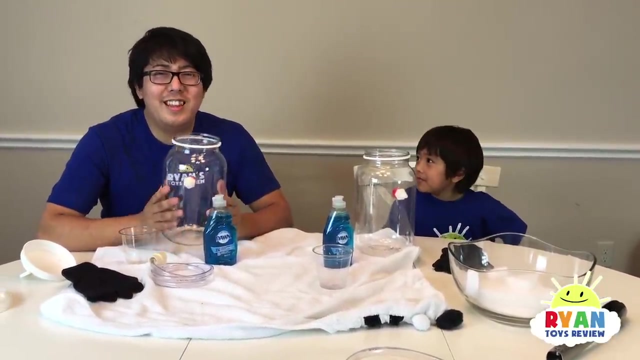 That looks so cool. Whoa, it's really coming out a lot. Hopefully you guys enjoyed the pumpkin science experiment. Bye Happy Halloween. Remember, always stay happy and rise up. Bye Happy Halloween. The dry ice poo experiment: Poo. 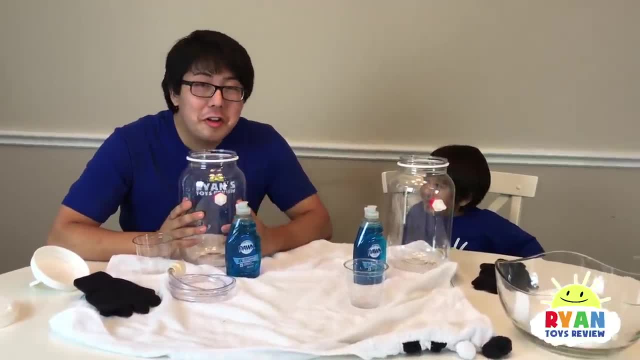 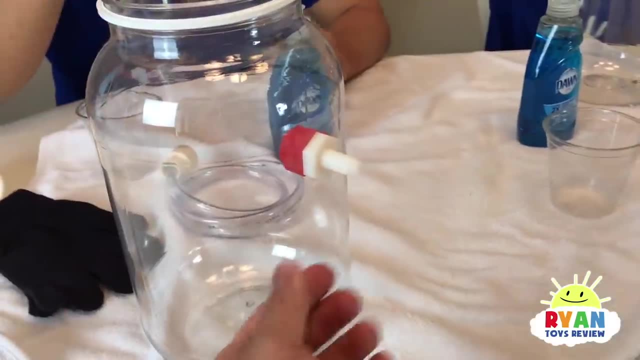 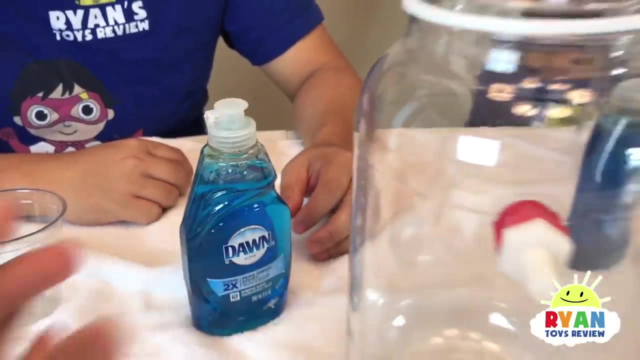 It's a scary bubble. A scary bubble, It's not scary, it's fun. So all you need is one of these containers here- You can make your own, but we bought ours- And then you need this hose to attach, And then you need some Dawn soap. 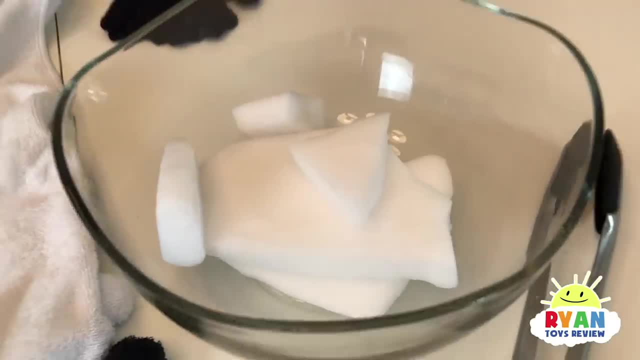 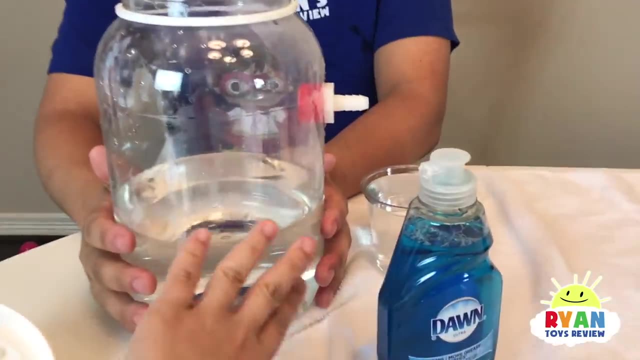 And then the dry ice, And then never touch the ice with your hands, so we're going to use these tongs here. So what we have so far, this is warm water in the big bubble generator container, And this is just regular distilled water. 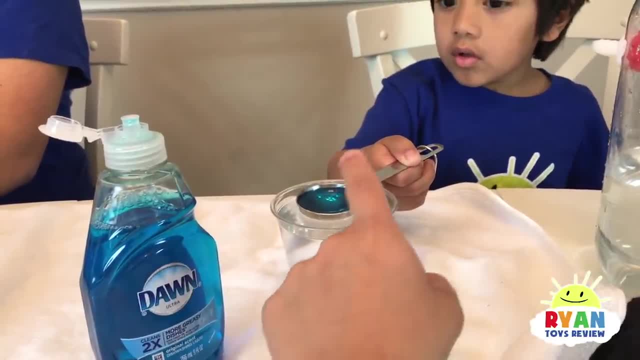 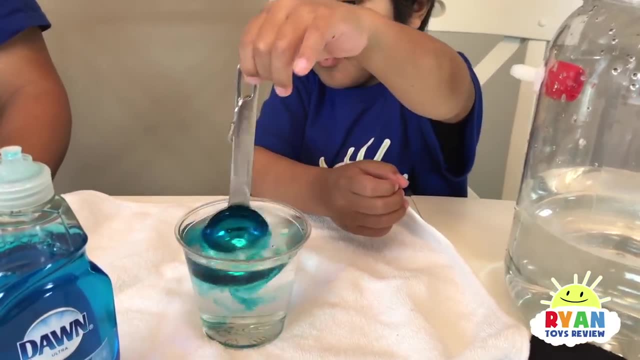 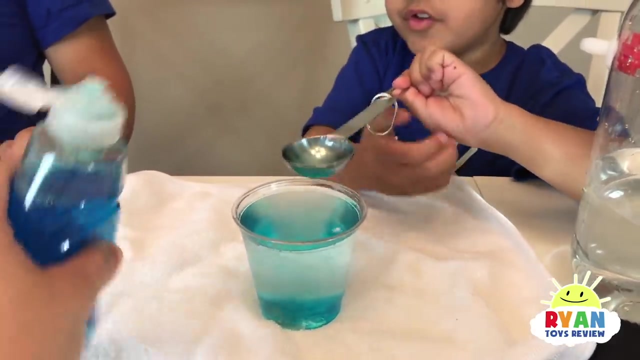 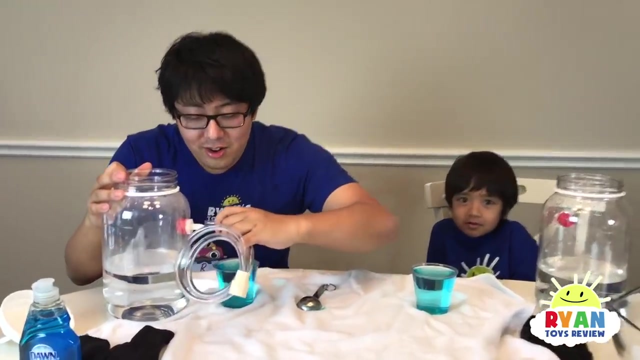 And here we have Dawn soap. So Ryan's going to put two tablespoons of Dawn soap into this smaller cup. Drop it. Ooh, Changing the color. there you go. There you go one, And we need one more. So attach the tube to the bubble generator. 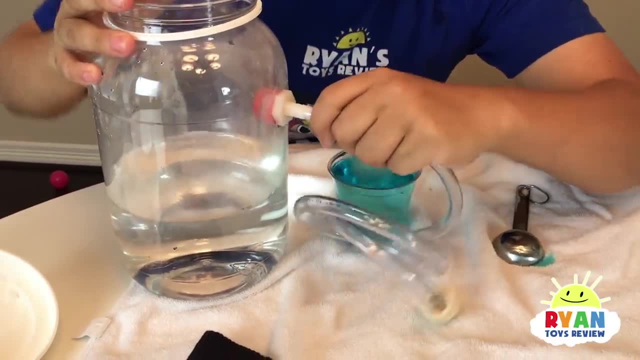 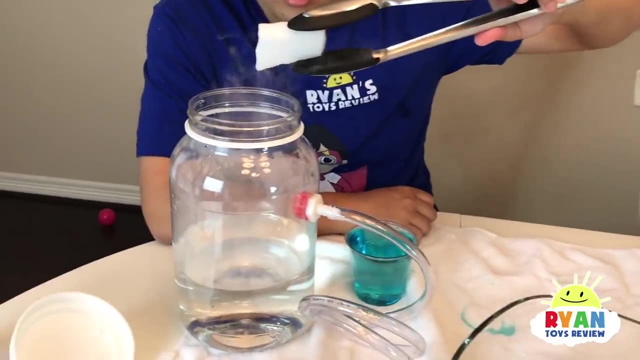 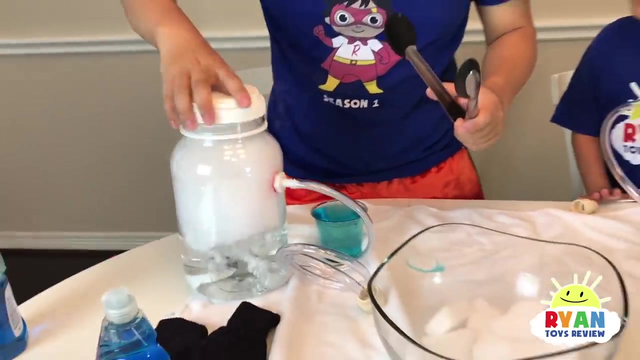 Push it really hard. Next, let's put the dry ice inside. So here it is. Never touch the dry ice with your hands and don't eat it or put it in your mouth. You want more? Yeah, There you go, Whoa. 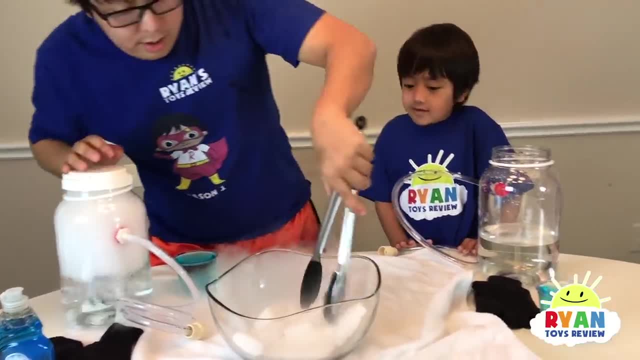 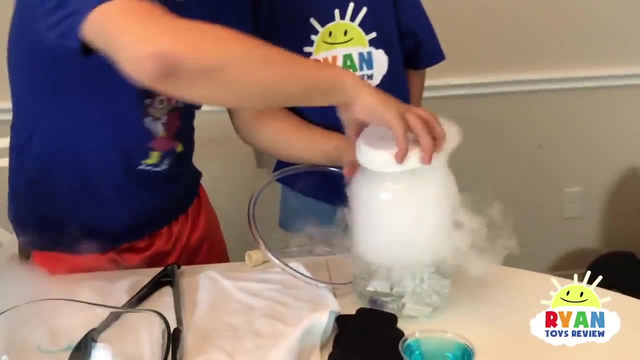 Clump it. Whoa, Can I do it to yours, Ryan? Yeah, do it to yours. Close the cap. Oh, it's so cool. Whoa, Open my mouth. I'm in love. Ah, Look, a fog's coming out. 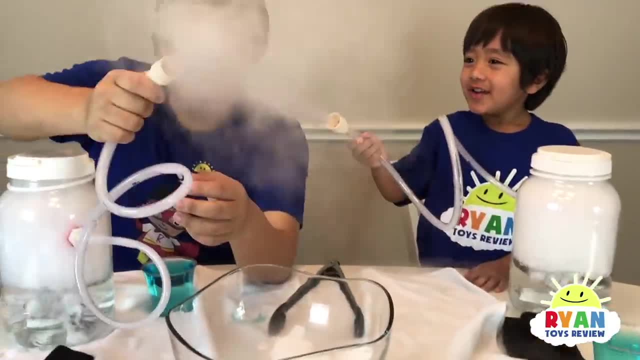 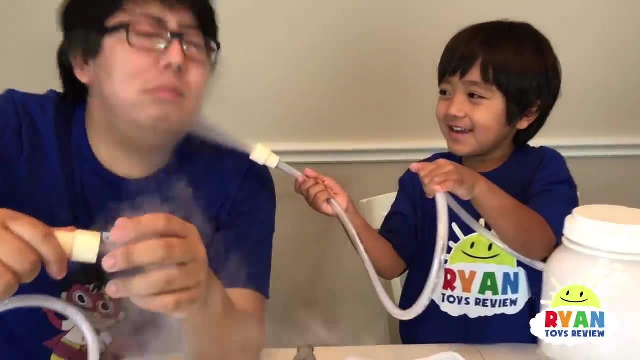 Ooh, Are you cold? No, Oh, yeah, that's a little bit cold. Oh, Oh, Ooh, that's so cool. Yeah, that is cold. Oh, That's cold. No, I'm just kidding. 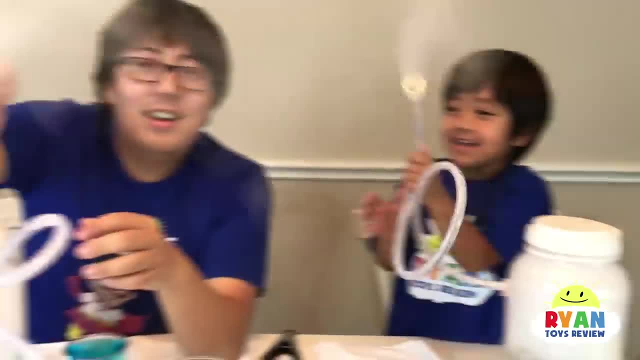 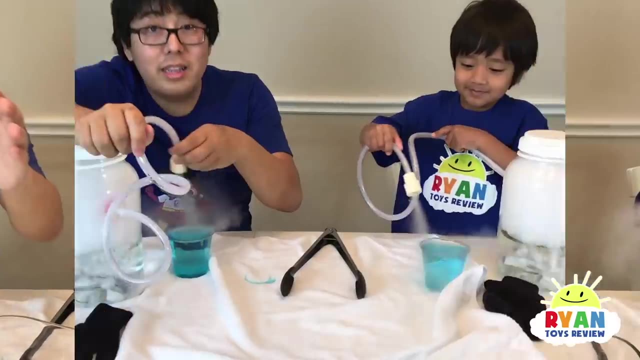 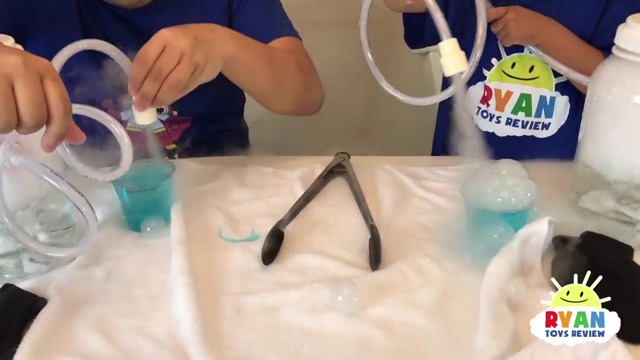 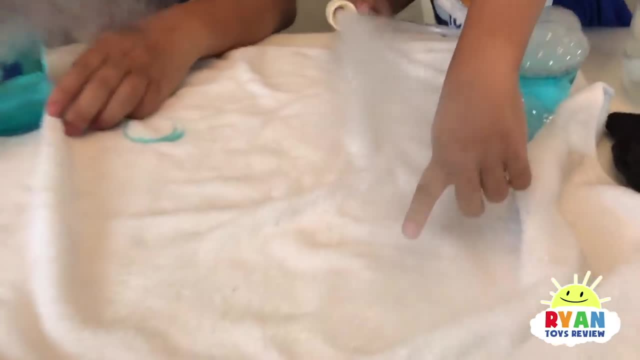 Boo bubble. Yeah, Ryan got his first boo bubble. Look at the boo bubble. Whoa. You have to do it faster with something You have to hold. Oh, I'm blowing. I'm blowing it, Whoa. Look at the boo bubble. 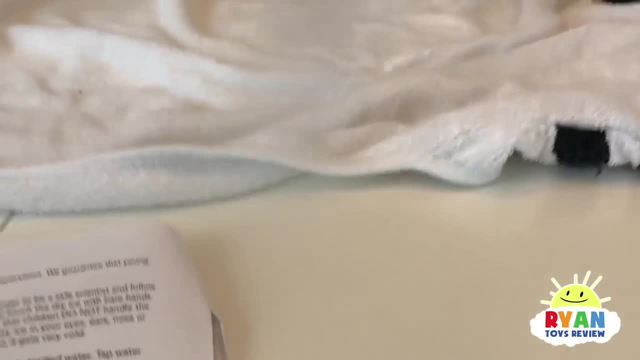 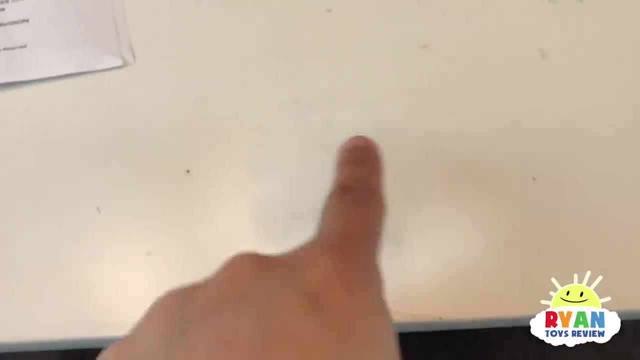 Whoa, Whoa, It's just the boing boing. Yeah, that's so cool. Let me touch the boo bubble. You can touch it, Ryan. Now you can touch it. It's just like bubbles. You can pop it. 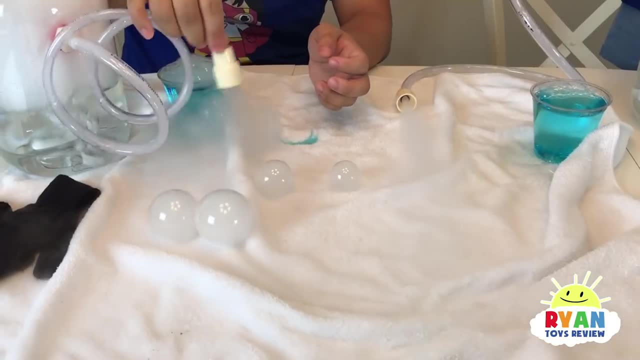 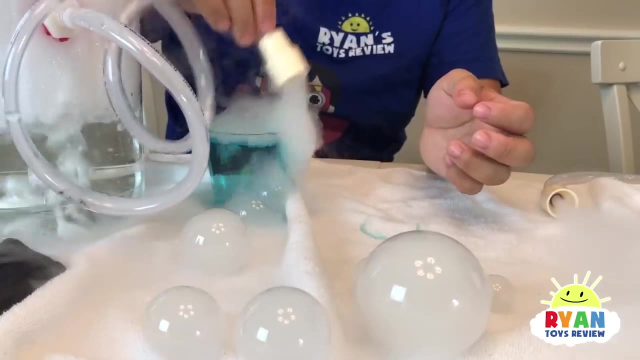 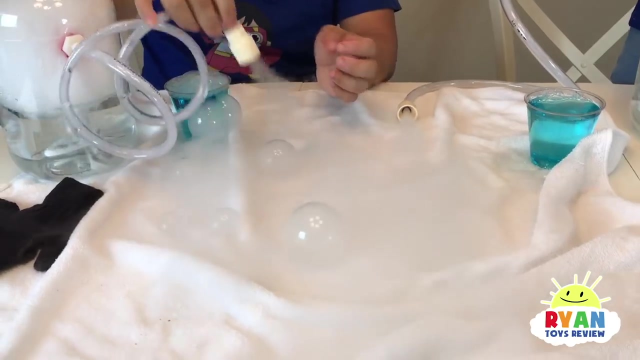 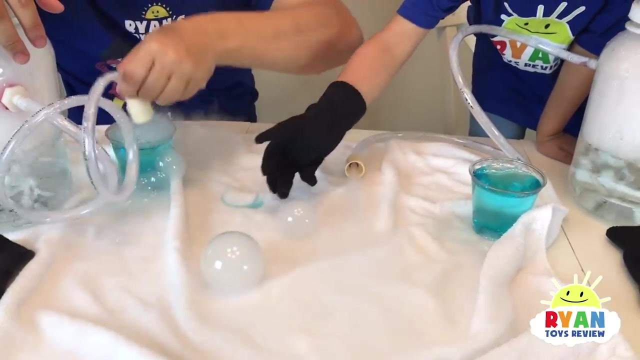 I want to pop it. I want to just hold it. Whoa, look at that. It's kind of a little bit tricky. Is this hard for kids? Wow, that's so cool. Put it on Ryan's hand, Okay. 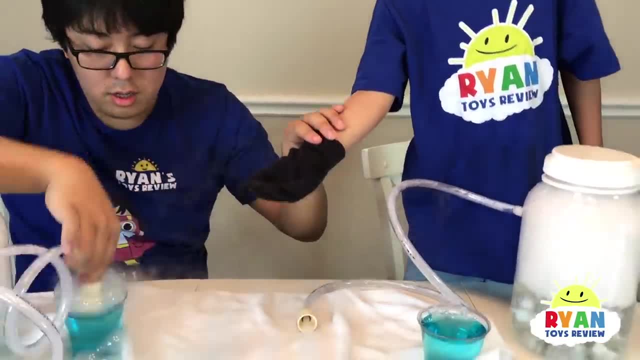 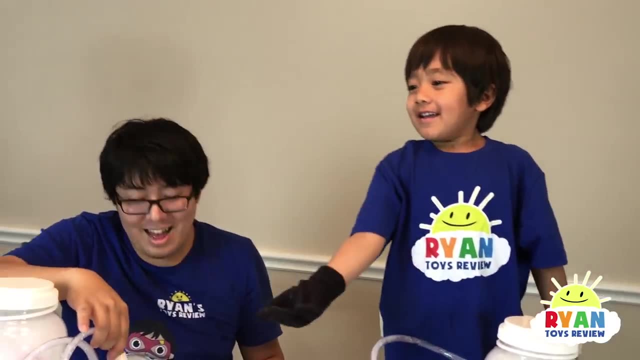 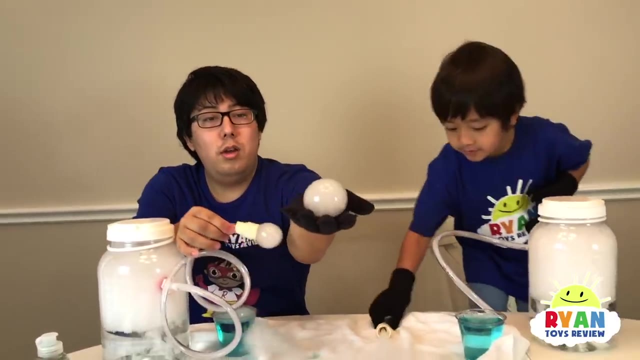 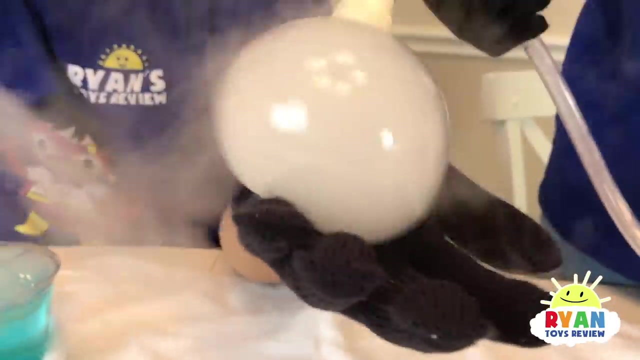 Put the glove on. Yeah, There it is. That's cool, That's funny. Whoa, look at that. Oh, I found a poo bubble, Your first baby poo bubble. Wow, look at Daddy's bubble. It needs a lot of air to pop. 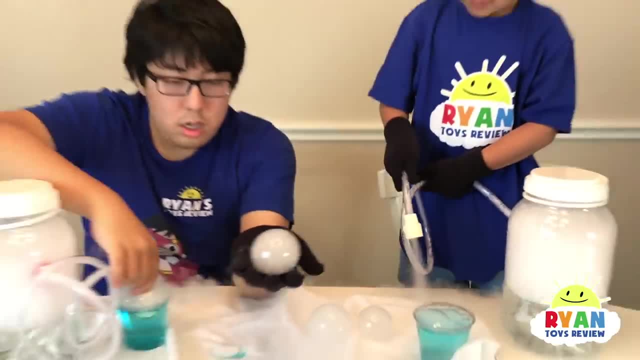 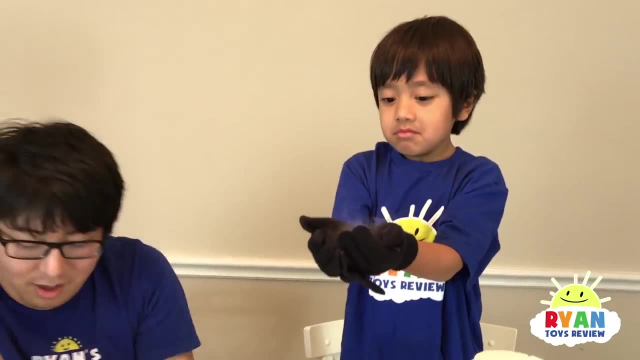 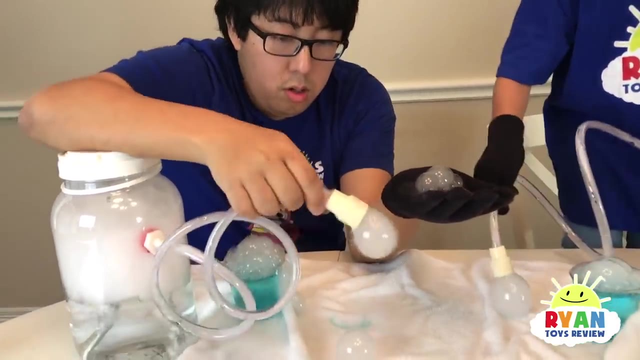 Ryan's poo bubble. Look at that. Okay, Whoa, Ryan picked it up. Yeah, Good job, That was nice. So usually regular bubble busts when they touch anything. So the bubble pops when they touch oil or dirt, But because it's on cotton it doesn't pop. 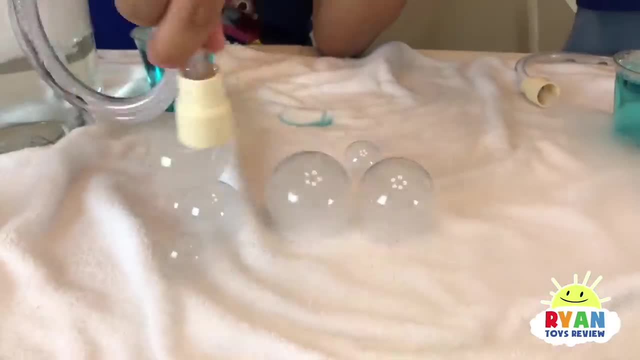 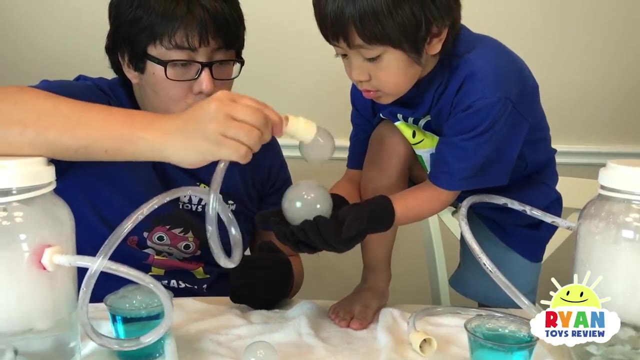 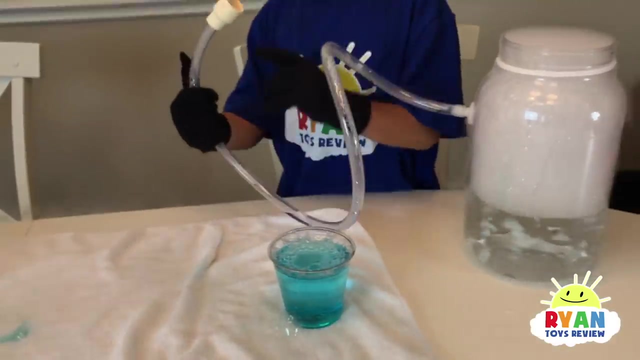 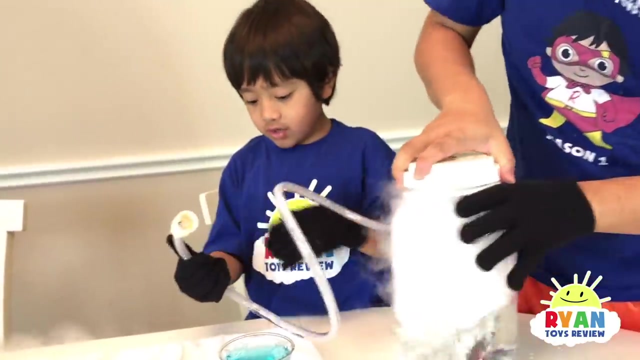 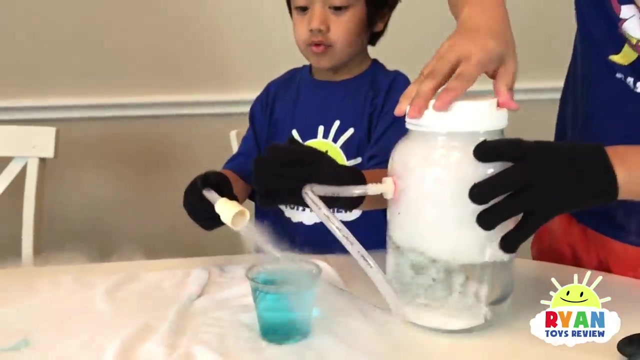 Look at that. That's awesome. Woohoo, What, Oh, Whoa, I don't want anymore Coming on the other end, It's coming. Whoo, Now I have more dry ice. Whoo equals Oh. 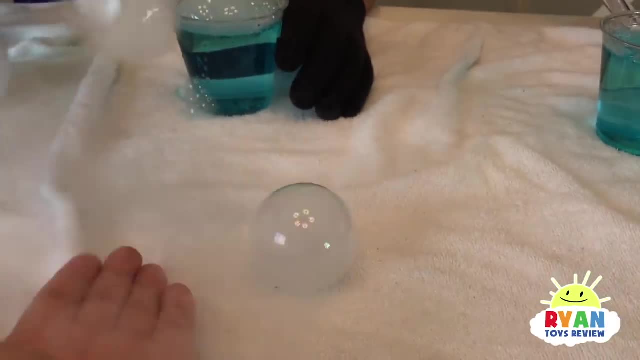 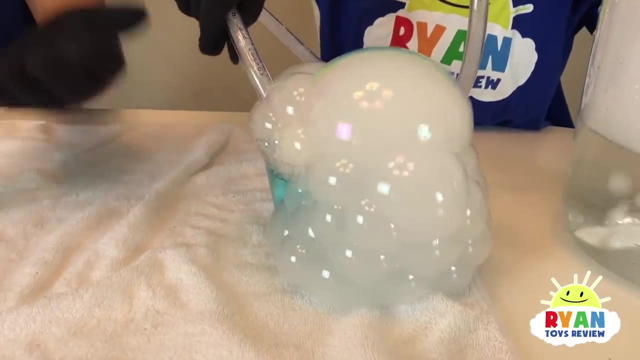 Tornado in the water. Yeah, Whoa, it's fun to pop it. See if you can connect and make a big boob bubble. Connect with him. Whoa, Ryan Daddy, Oh my gosh, Oh, a giant boob bubble. Whoa. 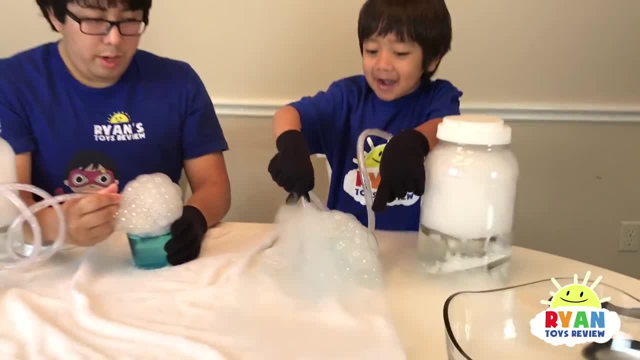 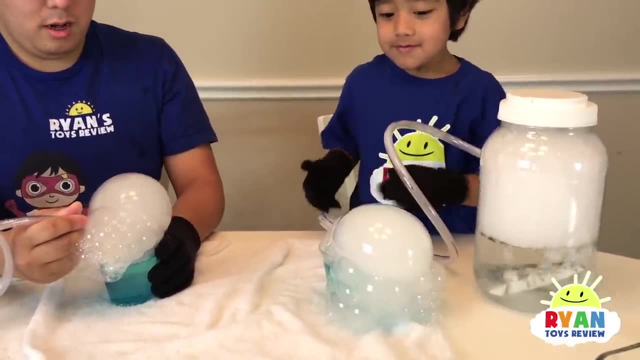 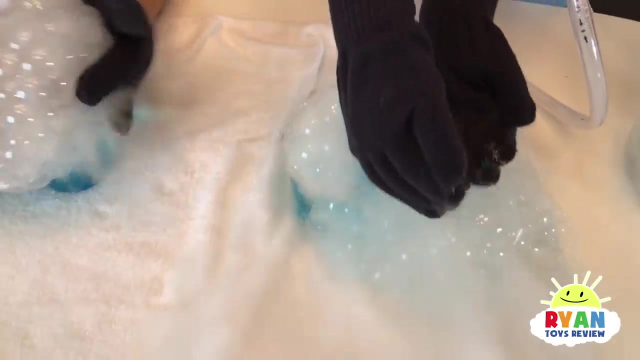 Look at that, Oh a giant boob bubble, Daddy. Oh my gosh Bubble explosion. Whoa good job, Ryan. Ooh, Whoa, Oh, I can touch it. Whoa Giant boob bubbles Funny. 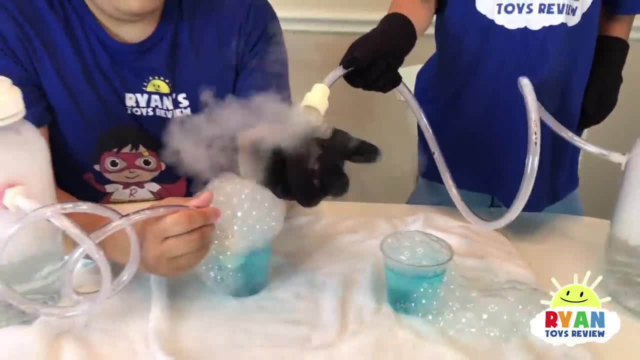 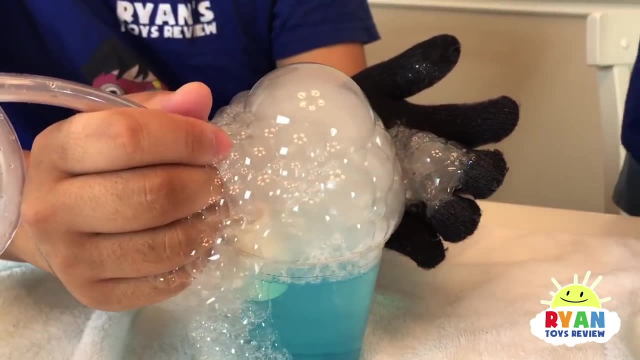 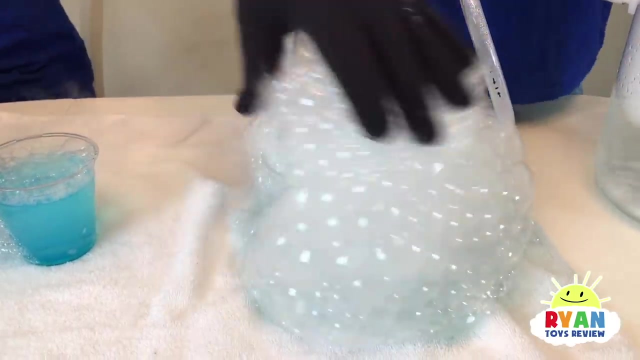 Whoa, They're cold. Wow, I'm amazed, Daddy, your bucket isn't filled. My bucket's filled. Yeah, it's a race, Ryan's winning. Daddy, Whoa, I can't even see the cup. Yeah, Where are you cup? 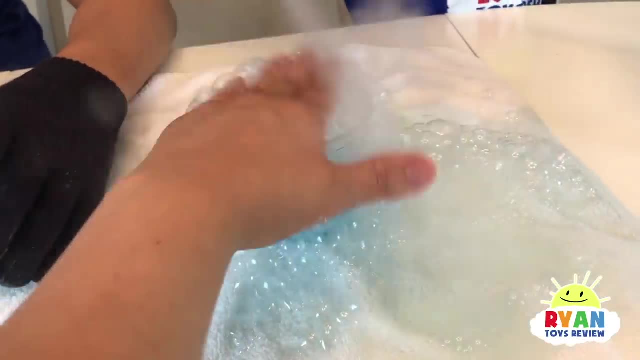 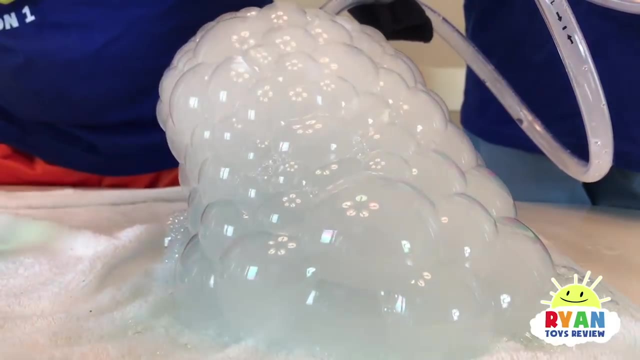 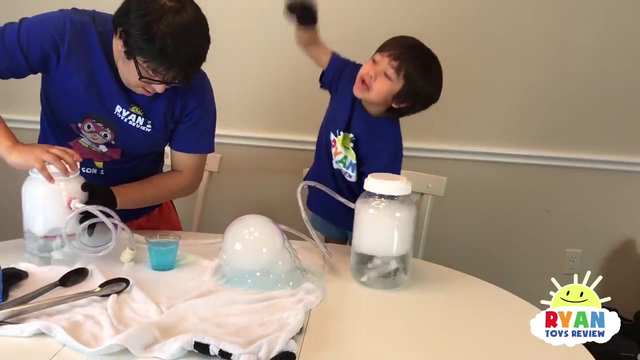 Whoa Still coming out. Pop, Pop, Pop, Pop, Pop. Wow, that's the wasp over it. Oh Look, I can see the light bulb up there. Yeah, Wow, Wow, that's the biggest boob bubble I've ever seen. 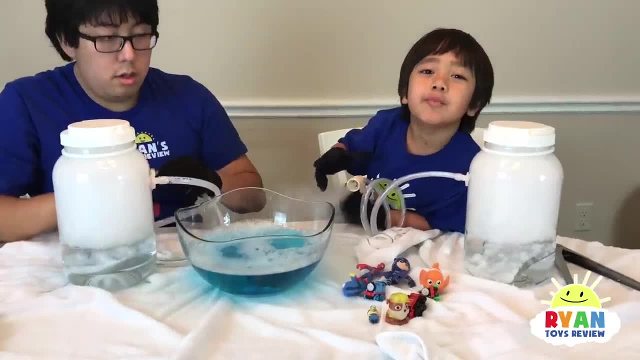 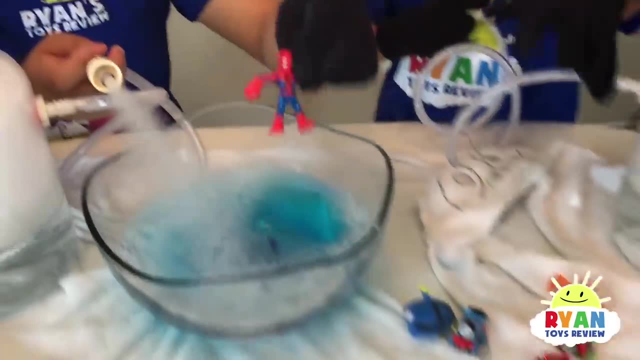 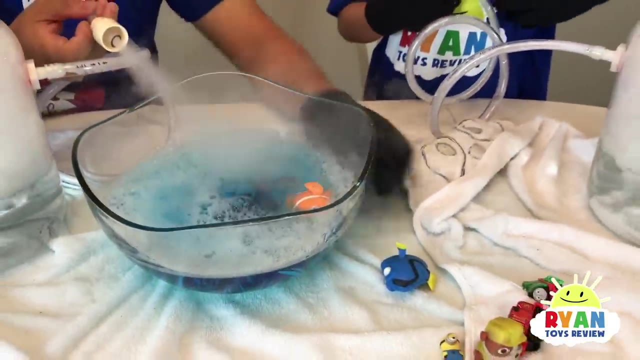 That's all the pops. yeah, That's cool. We're gonna put some poison for a swim. Ooh, PJ Mask. Ooh, Spider-Man, Spidey Nemo, Thomas Wait, Nemo's swimming. Everybody's not swimming. 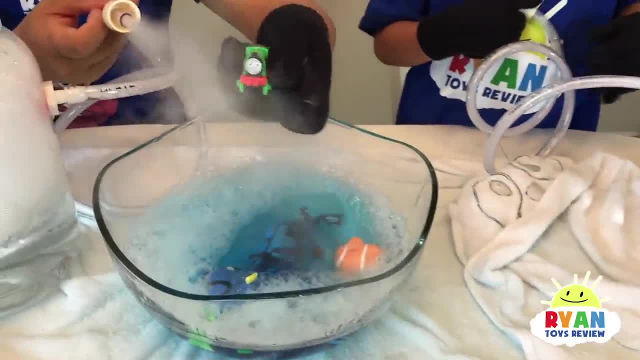 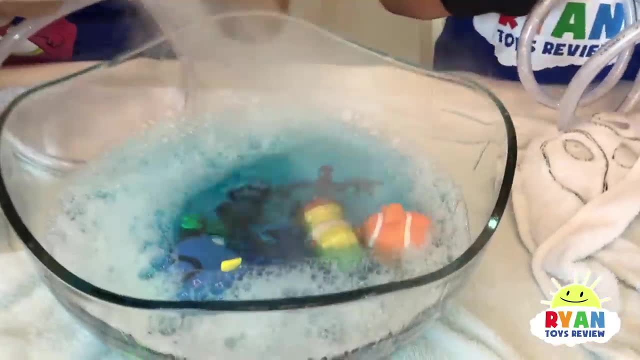 That's true, Dory, Dory, Percy, Percy. Who else Rubble? I think only Mashum's swimming James, James, Minion, I don't think he swims. Minion Woo, Let's put the hose in. 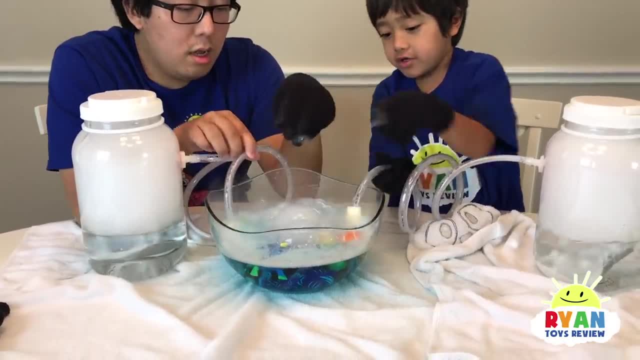 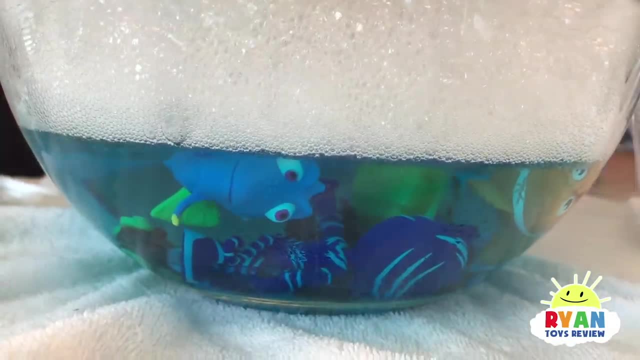 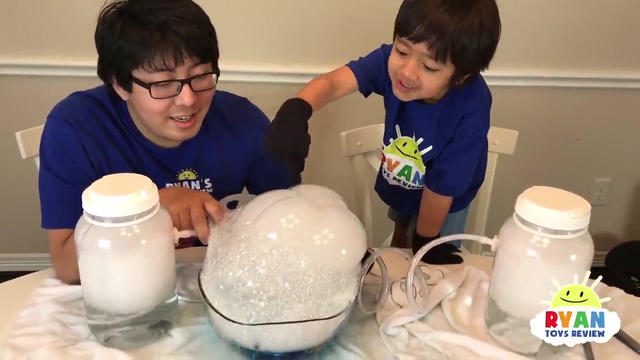 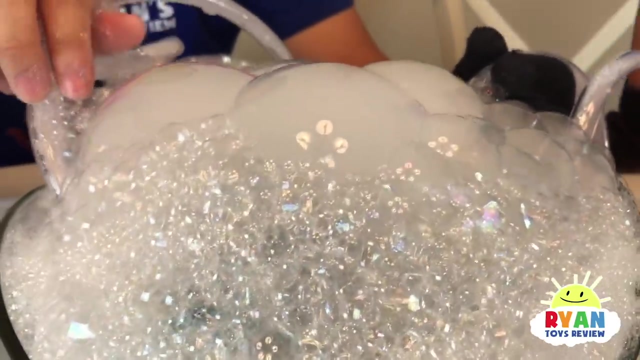 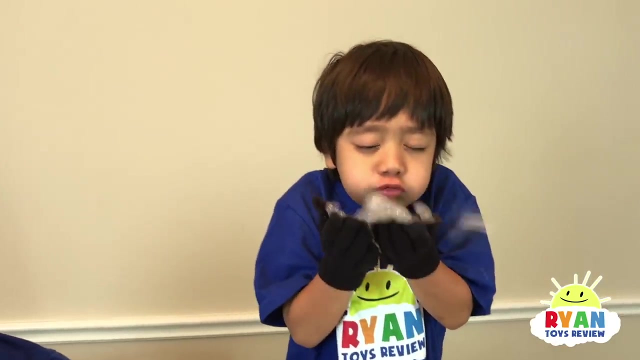 I'm locking it so it can be a long time, Okay, So I can put a lot. Well, that was fun. Woo, Okay, Okay, Okay, Woo-hoo, Ah, Woo-hoo, All right, so there, it is, Pretty colors. 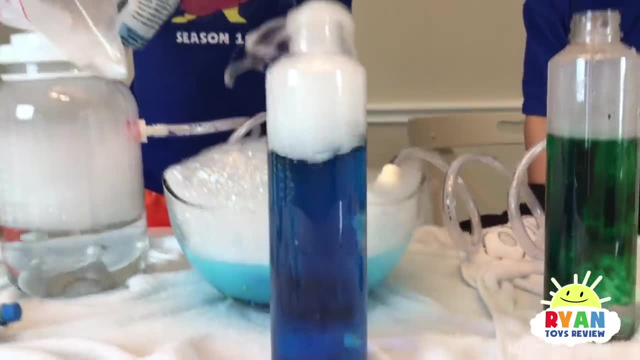 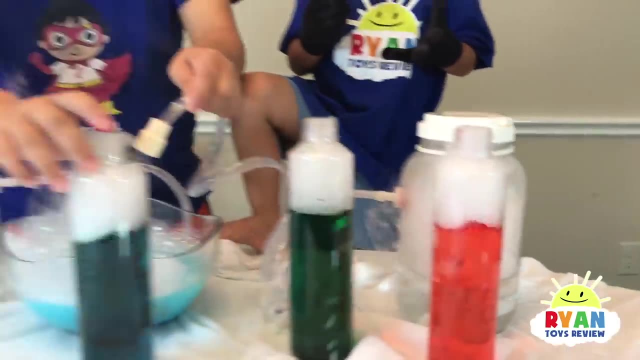 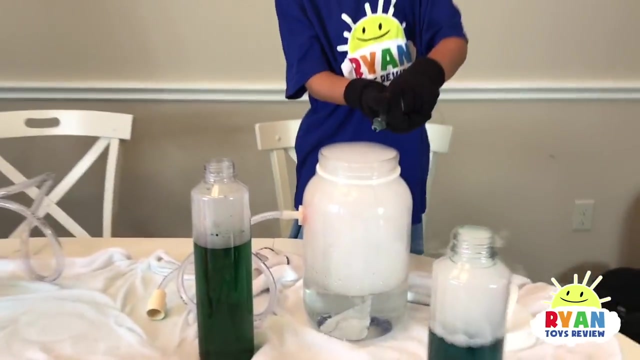 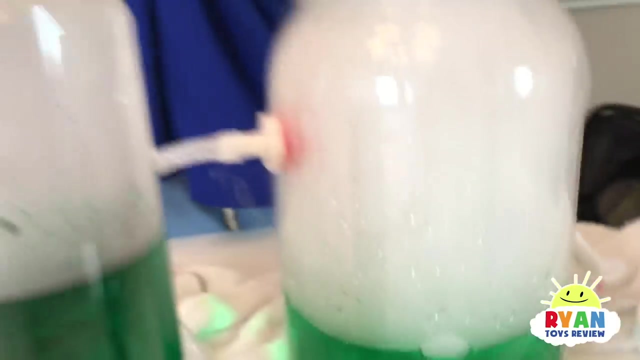 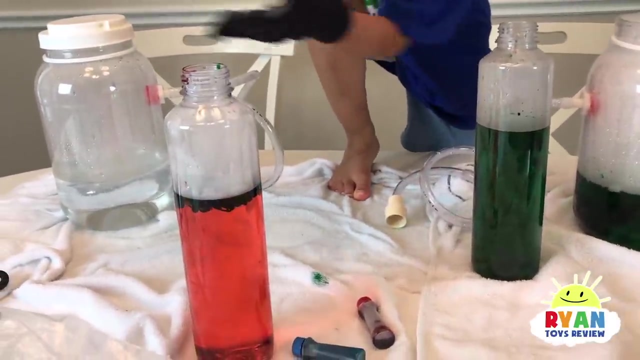 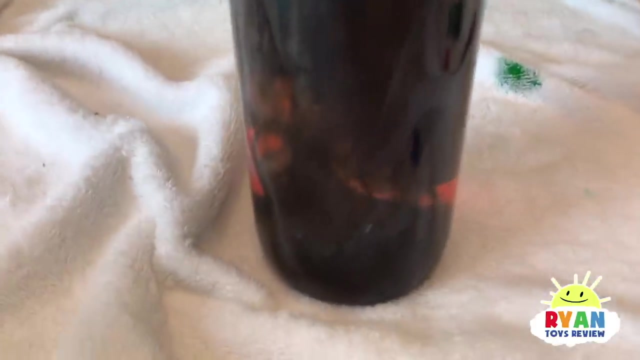 Whoa, I'm going to put three of these colors for fun. Oh, he just changed it to green, Woo-hoo. Okay, I think you put way too much green. now it just looks like black. look at that, too late. 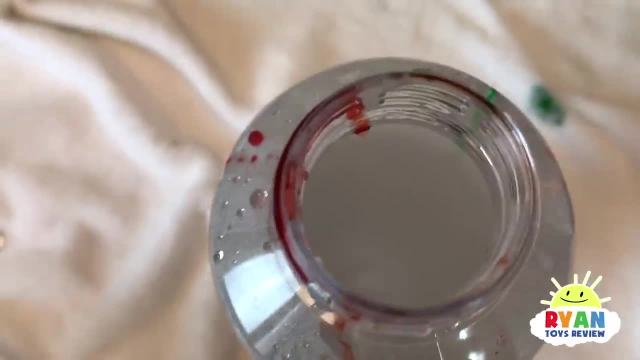 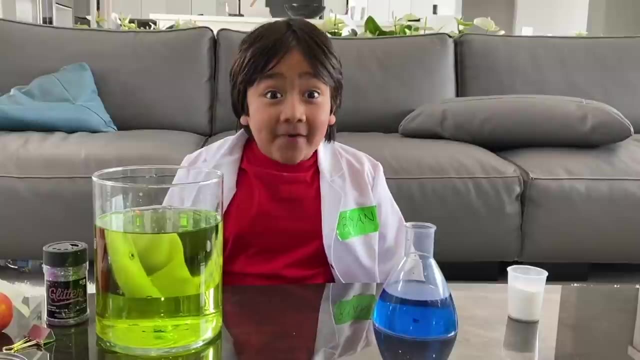 woohoo, Is it too late? Yeah, Hi guys, I know you guys are staying at home for a while, and I am too, so I'm going to show you some fun activities that you can do while you're at home. 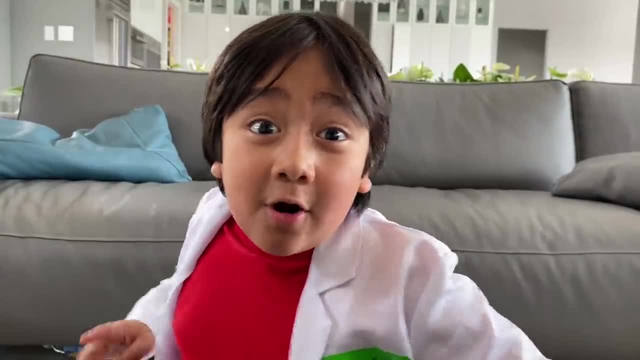 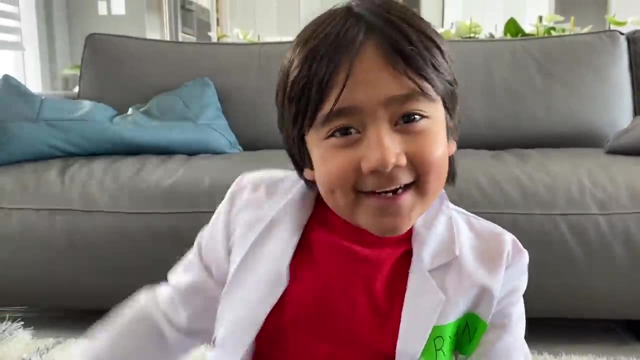 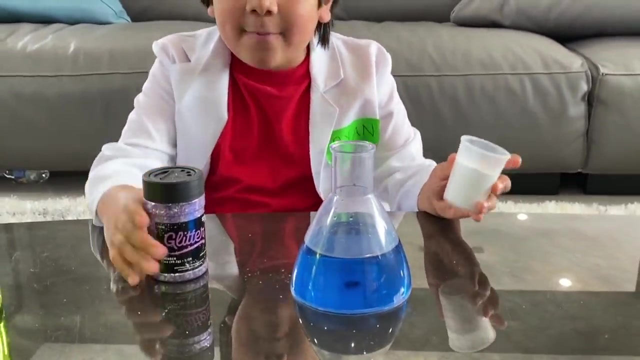 You can do all of these experiments, but remember, always ask a grown up for help. I've got my mommy here, hi. First experiment is one of my favorites- baking soda and vinegar- and we're going to spice it up a little with glitter. 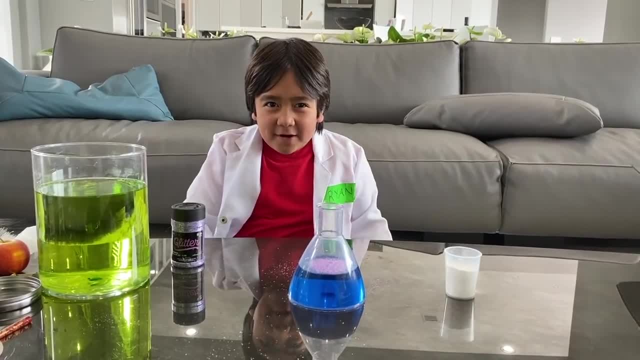 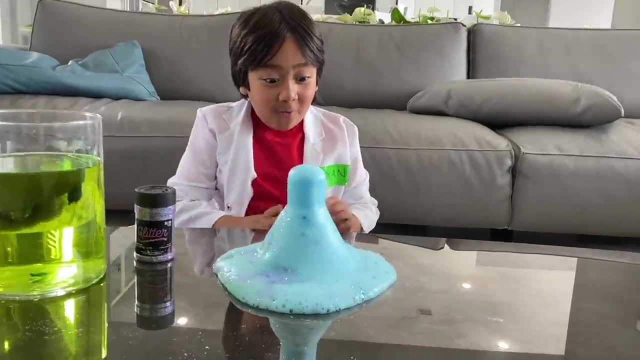 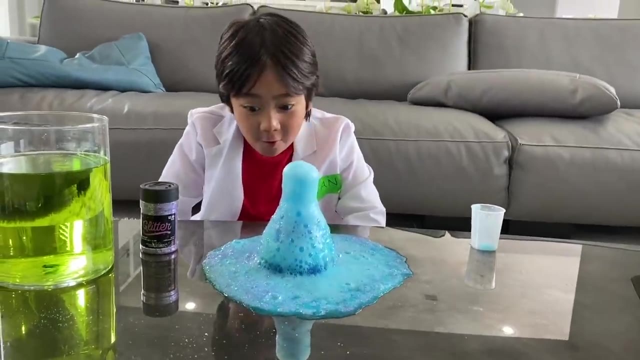 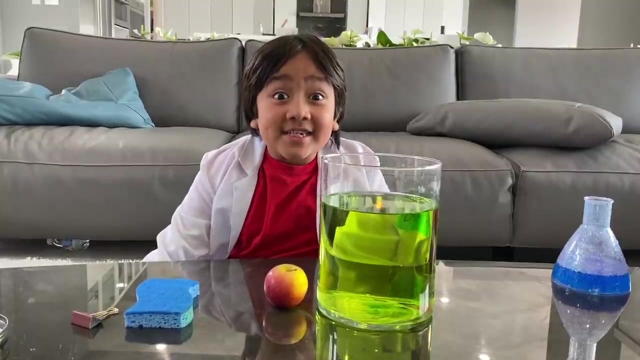 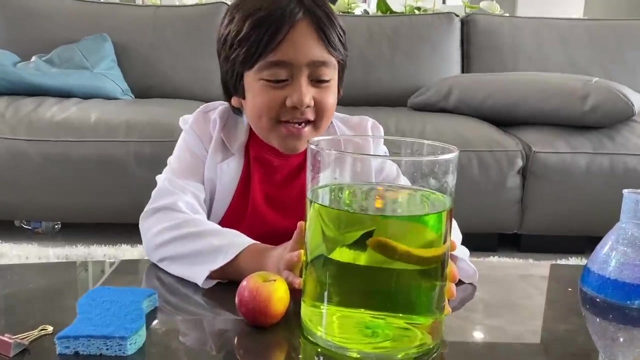 Get ready for an explosion. Okay, go, whoa, wait, I see all the glitter. whoa, that looks so cool, whoa. The second experiment is also one of my favorites as well. it's the sink or float challenge, because all you need is some water and some items around the house. 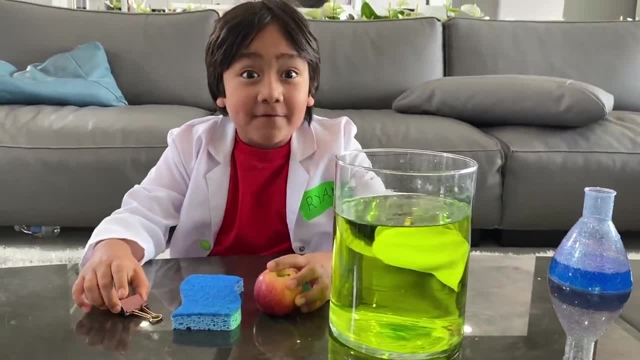 Okay, You throw it in and see if it sinks or floats. I think this one will float. Okay, It does float. What about this paper clip guys? do you think it's going to sink or float? Okay, let's see. 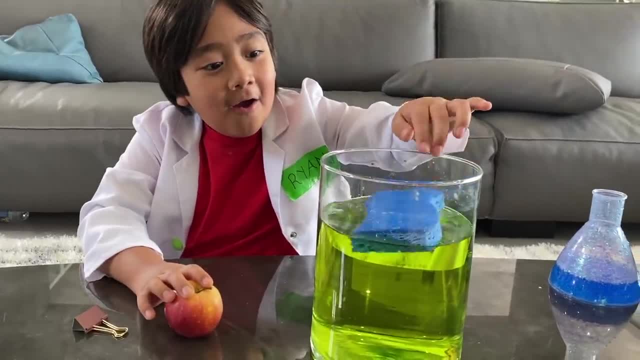 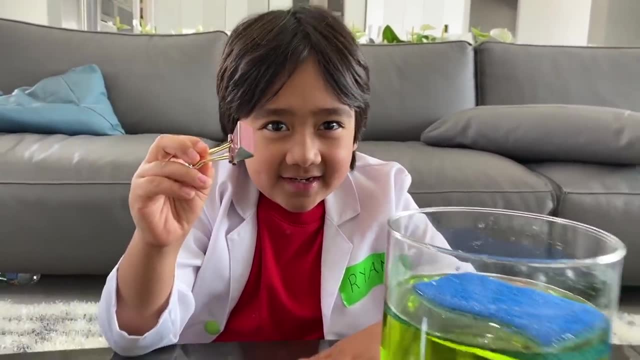 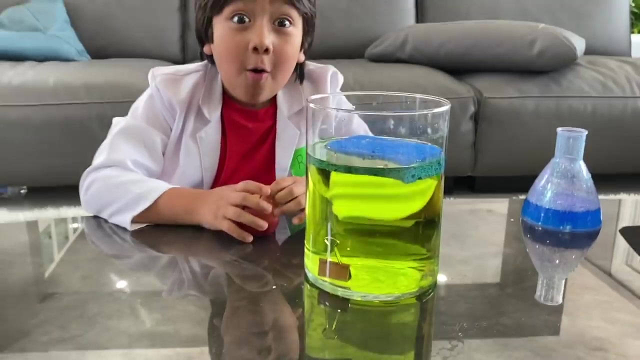 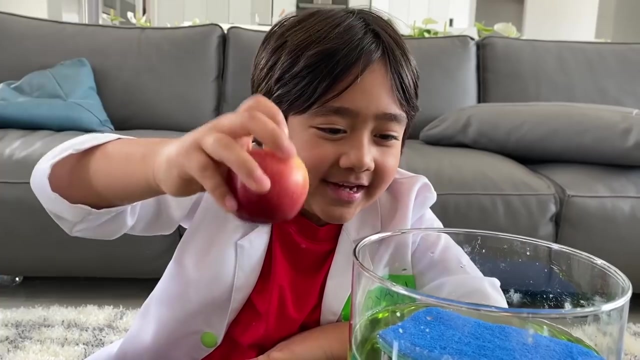 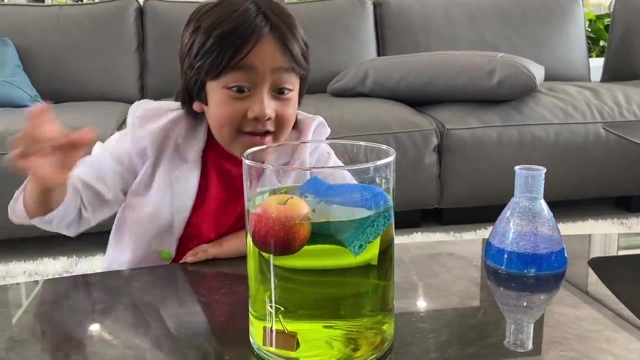 It sank all the way to the bottom. Whoa, Now let's try this apple. do you think it's going to sink or float? I think it's going to. maybe float. Yeah, it's floating. So two of them float and one of them don't. 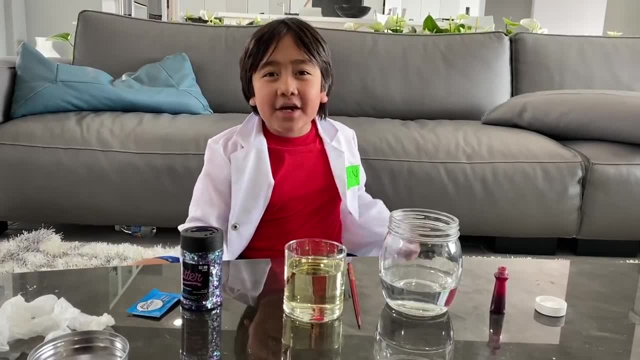 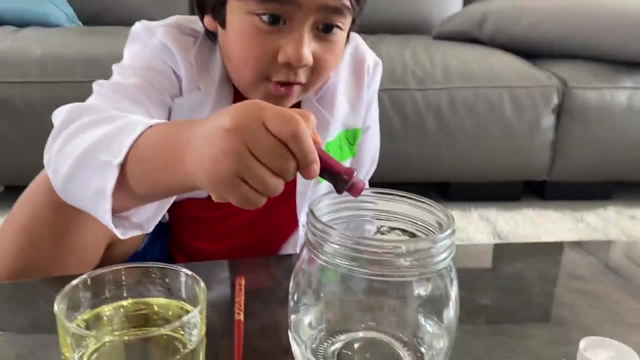 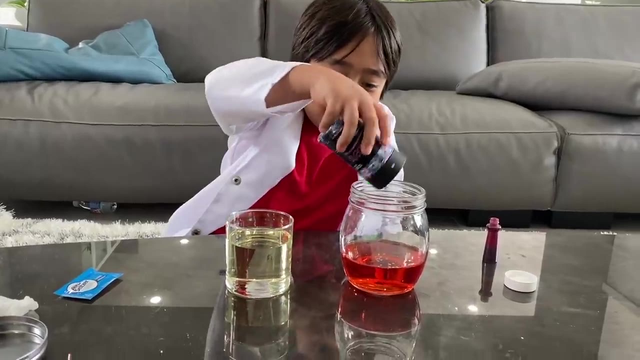 Third activity, also one of my favorites: the homemade lava lamp, and it's easy to make. All you need is food coloring, one drop of water. Okay, Then agitate, agitate, agitate, agitate. Optional glitter, of course. 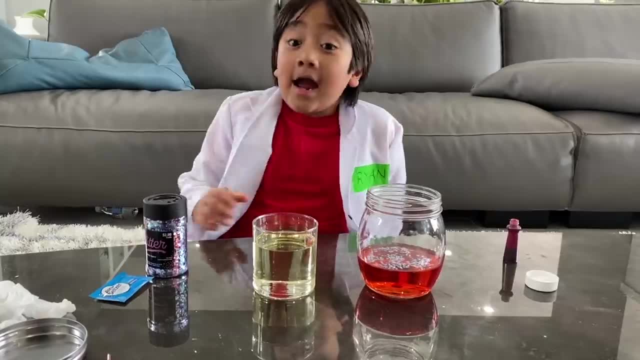 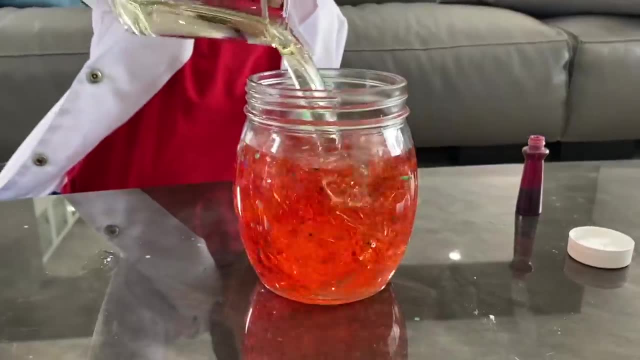 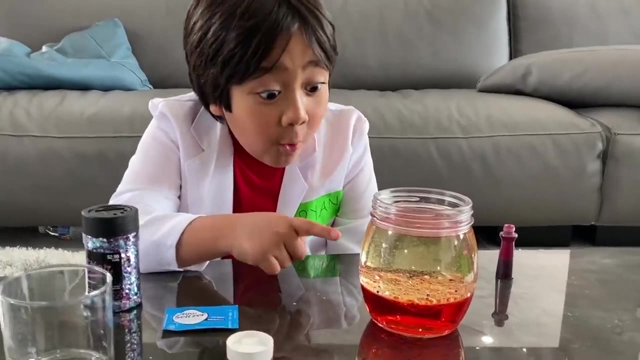 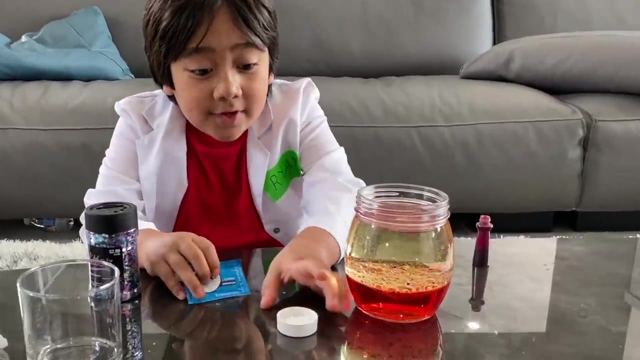 Okay, Next some vegetable oil. Ooh Whoa, Do you see how the water and the oil is separated? That's because they have different density. Next up is some broken up Alka-Seltzer. I have some right here. 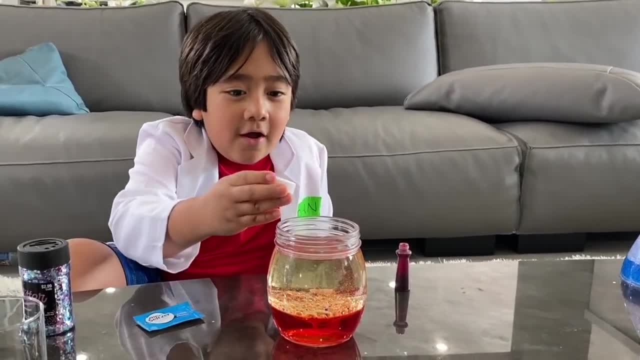 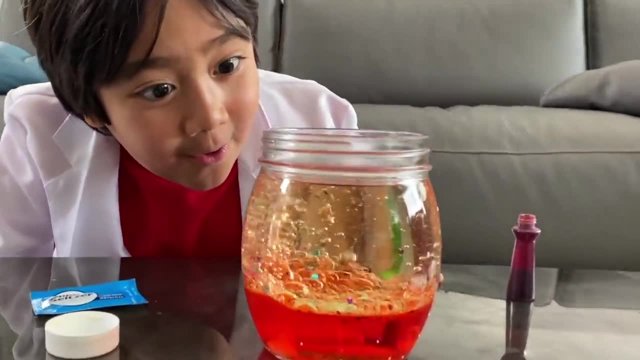 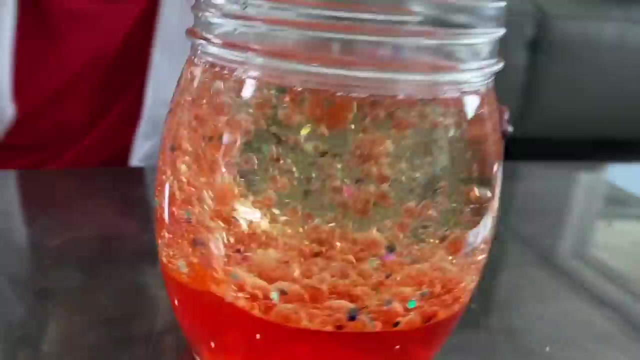 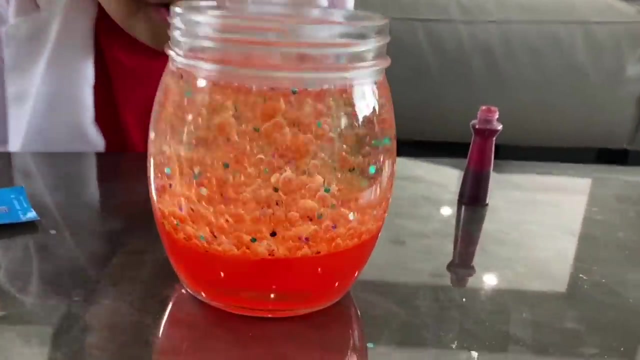 Okay, Three, two, one, Go Whoa, look at it. Ooh, that looks cool. All of that's going up there. Ooh, It's like, ooh, ah, Wow, this was so much fun. 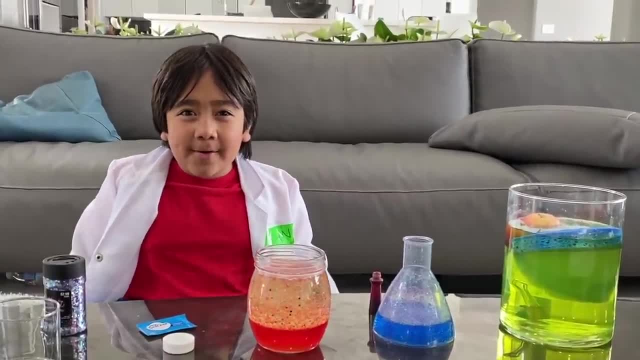 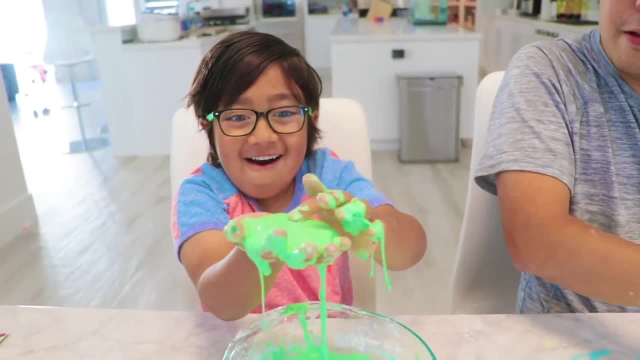 Here's some other science experiments you can do while you're at home. Have fun. Roll the science experiments that you can do at home. Whoa, How to make oobleck. Hi guys, today we're gonna be making oobleck. 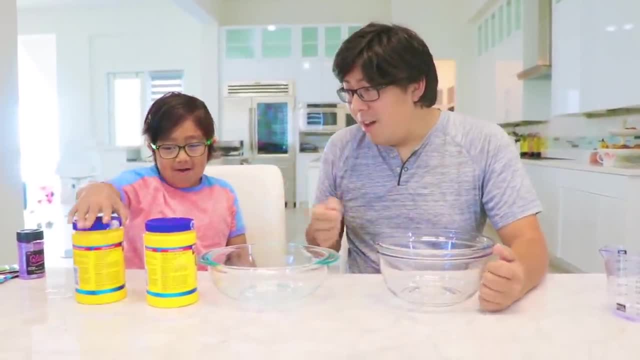 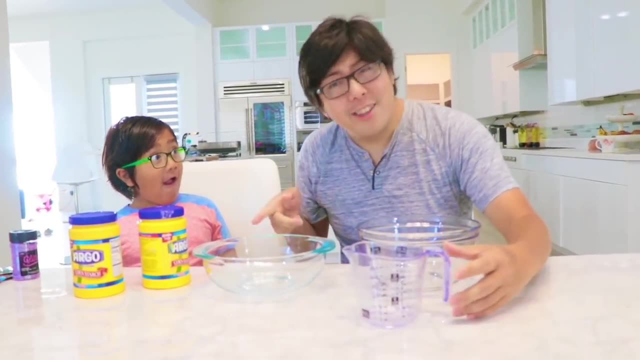 with cornstarch and water. Whoa First ask a grownup for help, Which is me All right. So first we need 1 1⁄2 cup of cornstarch. Okay, Ryan, open it up. 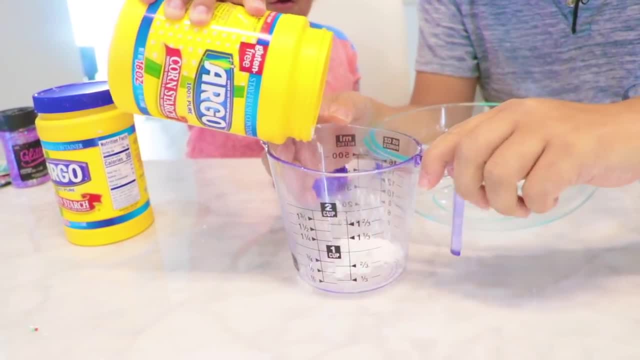 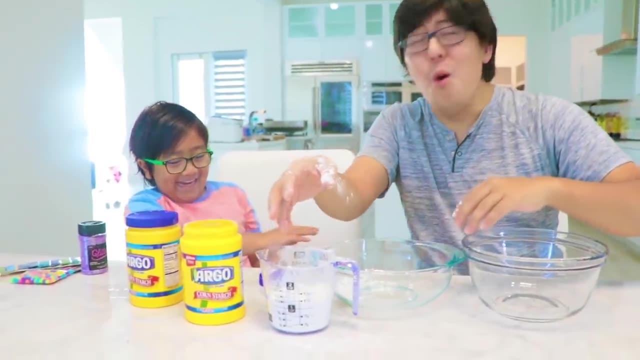 Start pouring it here. Good, more, more, more. Do you see the line where it says 1 1⁄2?? Ooh whoa, whoa Ryan, too much. This is why you need the help from grownups. 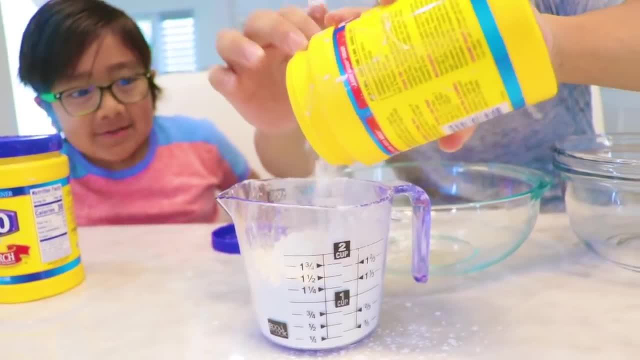 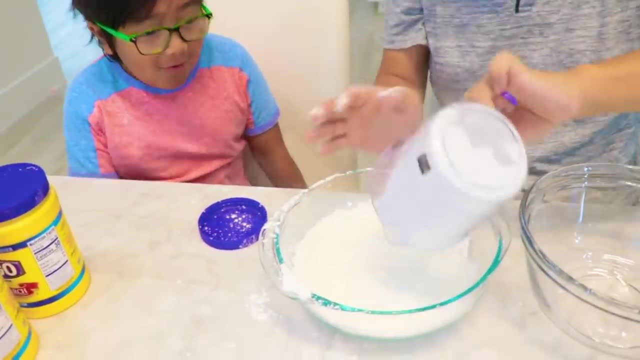 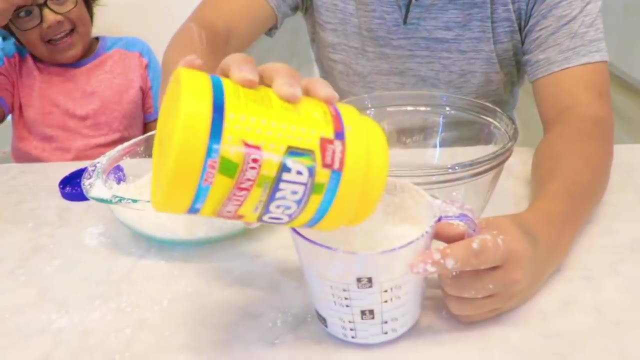 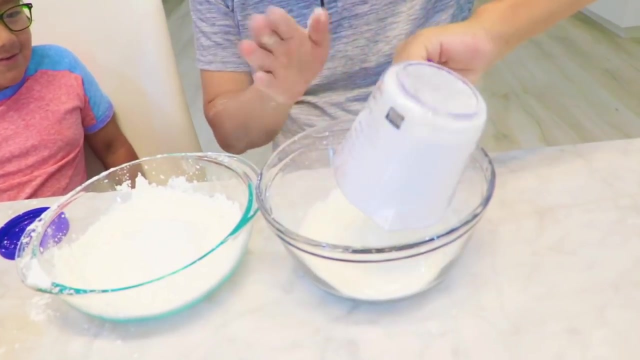 Now pour this in here: Doo, doo, doo, ooh. Oh, It's already getting messy For me. I'm gonna do the same thing. Wow, It's like flour, Yeah nice. You know never to eat anything. 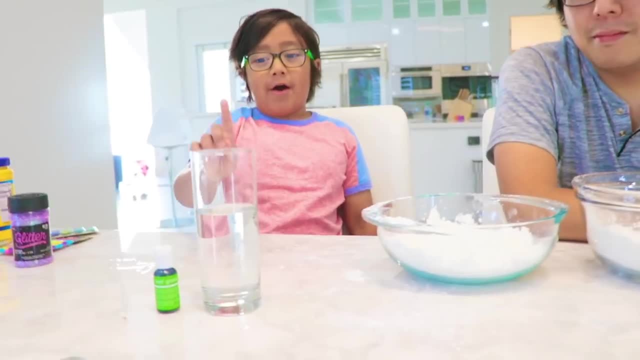 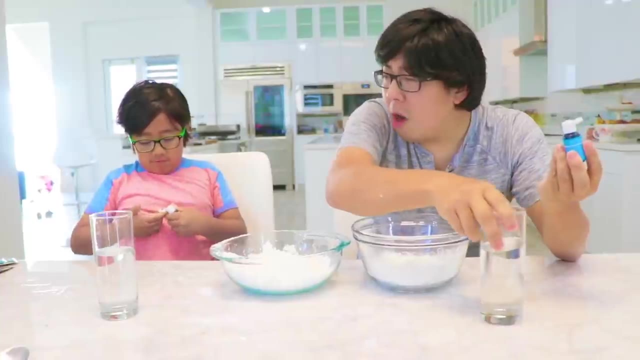 when you do an experiment. Next, measure out one cup of water. I'm gonna use green and Daddy's gonna use blue. All right, that's my favorite color. Okay, Three drops is enough, Ryan. Yeah, If you do too much, it's gonna be too dark. 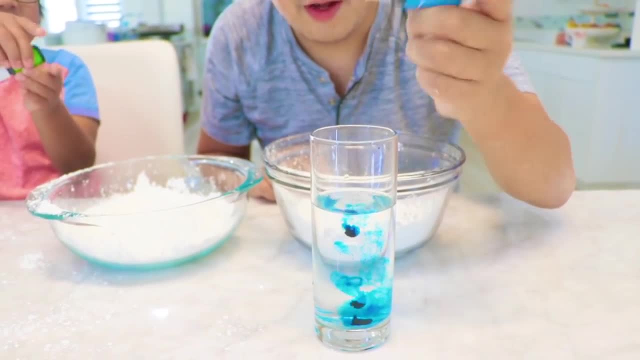 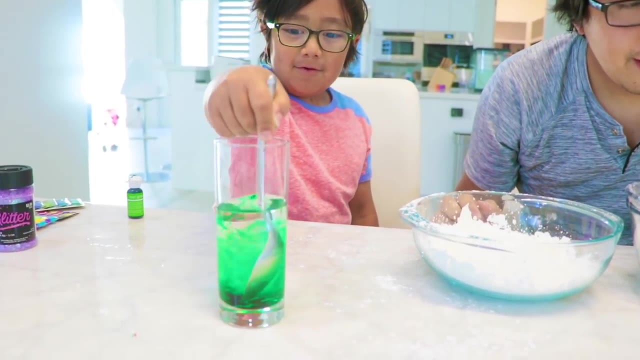 So one, two, three, I think that's good, All right, One, Oh, That's good, That's good, Just stir it. Ooh, these are big Whoa, look at that. Mine's definitely blue color. 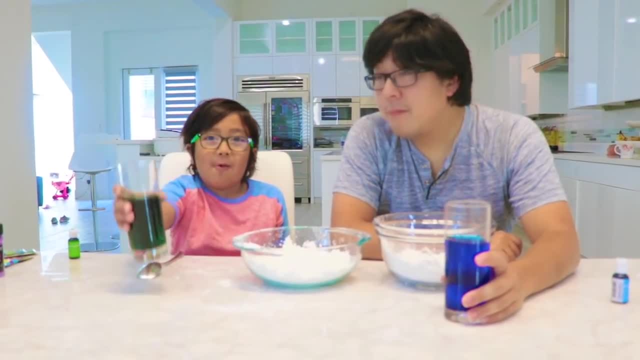 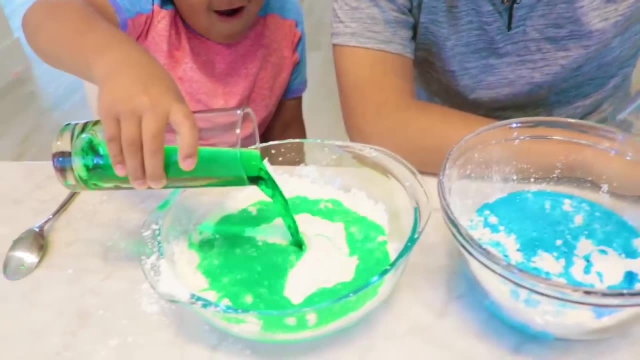 Whoa, How's yours going? Oh, nice, Nice green. Next, put the water into your corn starch. Whoa, Whoa, Whoa. Looking cool, Whoa, Whoa, The color came out. nice, It's like a volcano. 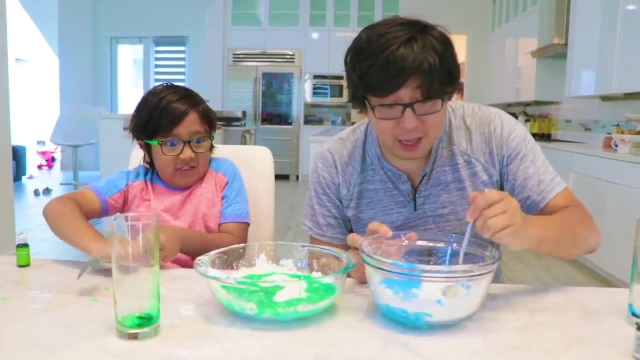 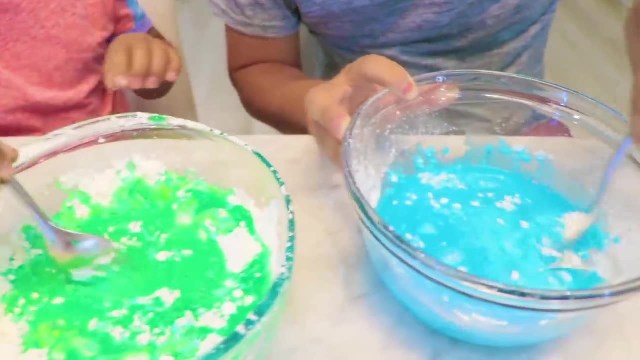 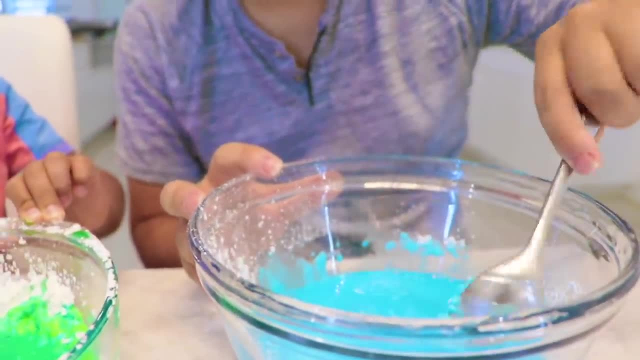 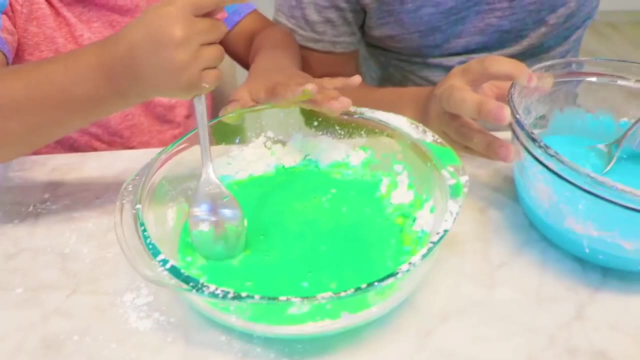 It's gooey. I love the color of mine. It came out really cool. What? Yours looks like soup. It looks like slime. Yours looks like a slime color. Yeah, Oh, it's plus on me. If you guys like messes, you should definitely make one. 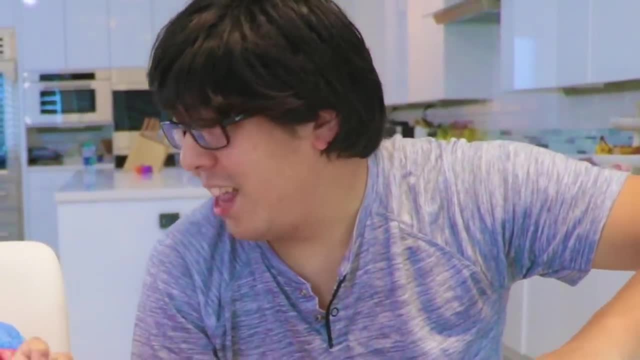 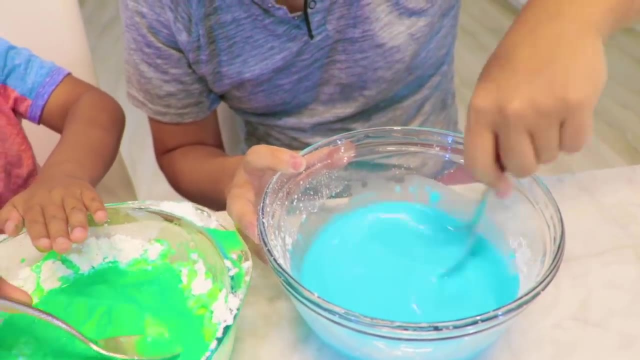 Yeah, I do, but. But don't make a mess intentionally, okay, Don't do that on purpose. It's all dissolved, I don't feel anything anymore. It's all liquid. I feel so much. This is why you need the help from the grownups. 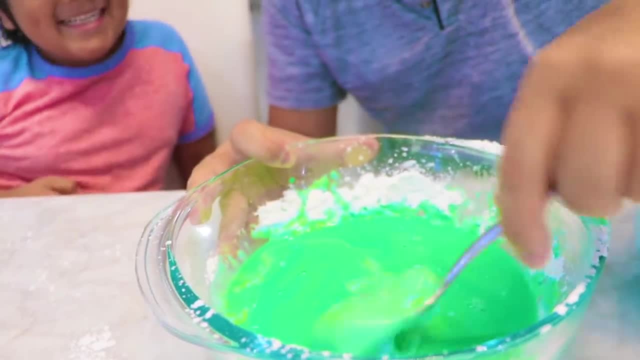 Whoa, Whoa, Ooh Ooh. Look at this big chunk. If it's too liquidy, you can add more cornstarch. Mm-hmm, I think mine needs a little bit more. Mine's good. 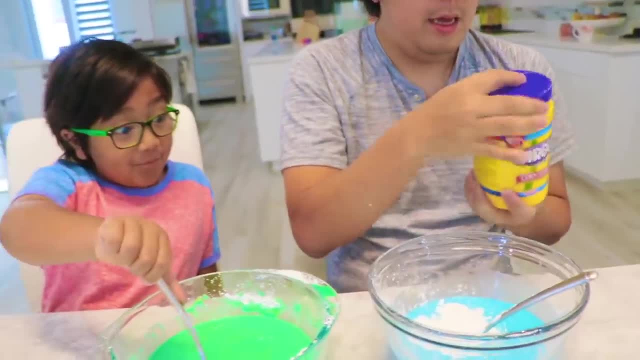 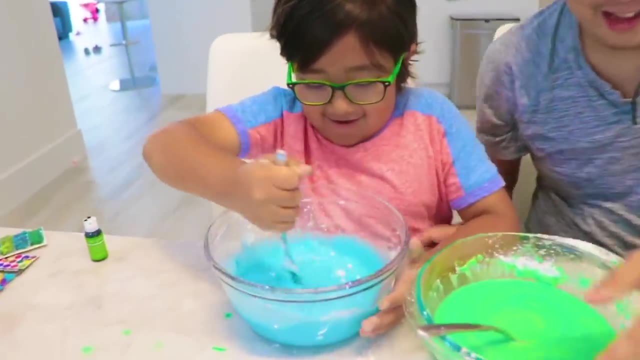 Yours good, Okay, Yeah, I'll just add a little bit. Okay, that should be enough. All right, We exchange. Here, you help me and I help you. Here you go. Oh yeah, Ryan needs a little bit more too. 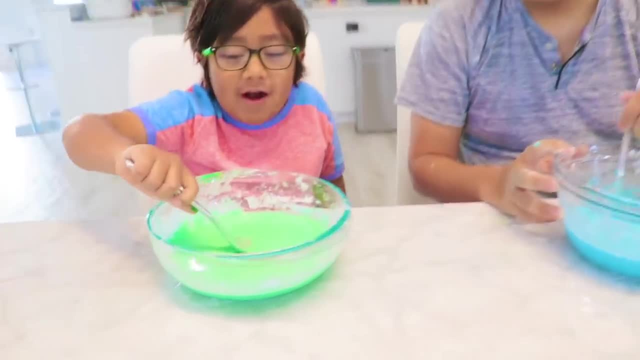 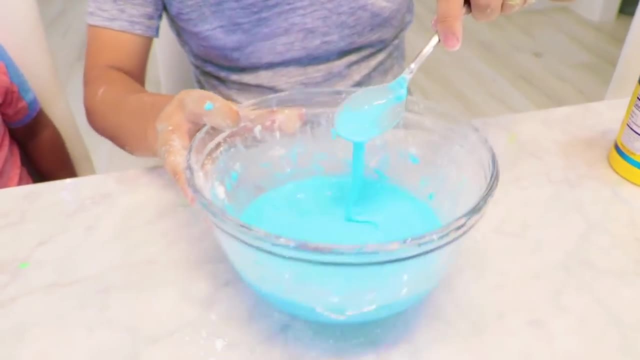 Look, It's very liquid. You know it's ready when it feels hard Like this. Oh, That's definitely ready, And mine too. Look at this, It looks liquid. right And Come here, Slap See. 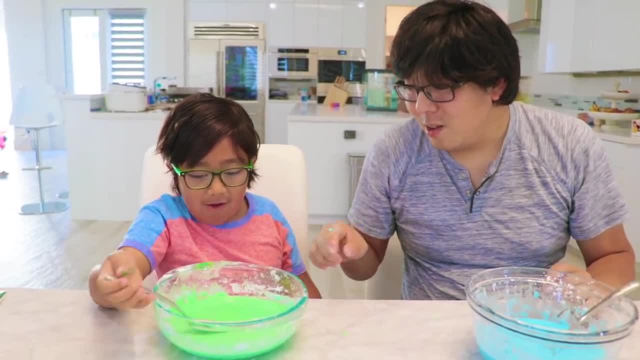 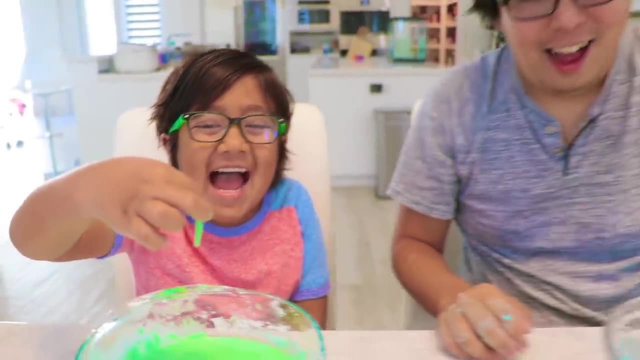 You can slap it. All right, Ryan, Why don't you try and touch it and see what it feels like? Oh, Whoa See, if I try and slap it I can punch it. See, My hand doesn't go in. 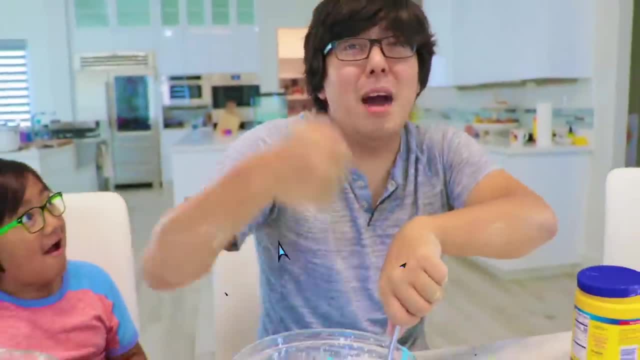 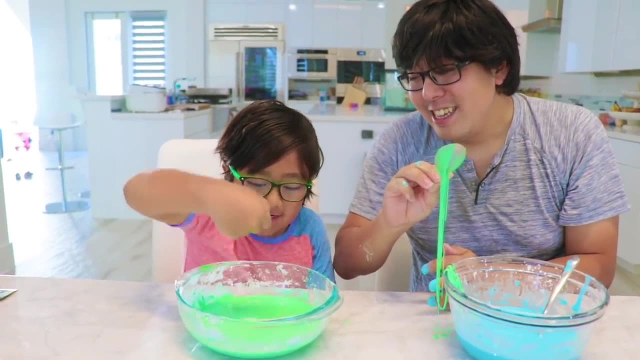 Look, Ah, can't punch through. Whoa, Let me try. let me try See What. So it's like slime, like that. It's kind of like slime. It's like concrete. It's like slime that's not ready yet. 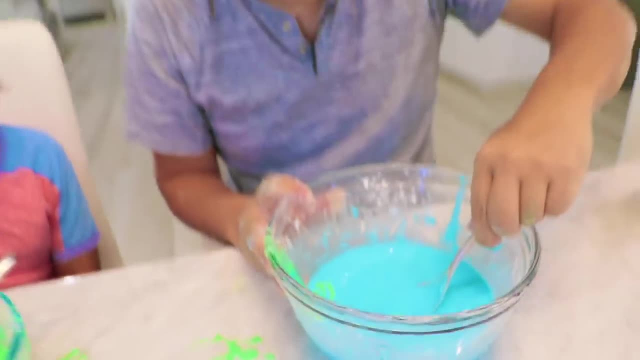 Oh no, I dropped mine. Oh my mine, No. So, guys, I have a question for you. What Is this oo black? Is it a slime, Is it a solid Or is it a liquid? It's both. 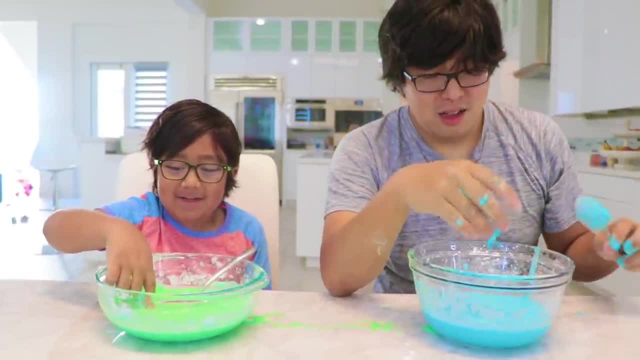 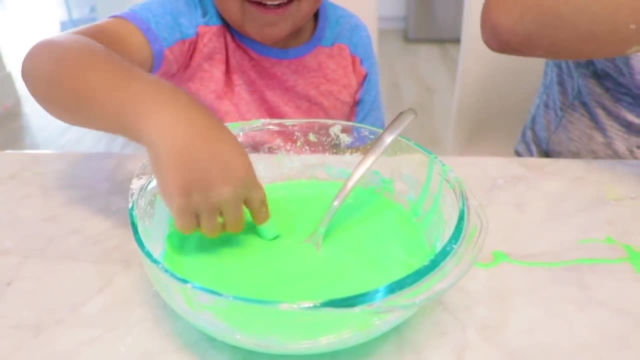 Why do you think it's both? Because when you stay still in it, it like sinks you down And whenever, whenever you hit it, it's a solid, So it's like invincible. Oh, I don't think it's invincible. 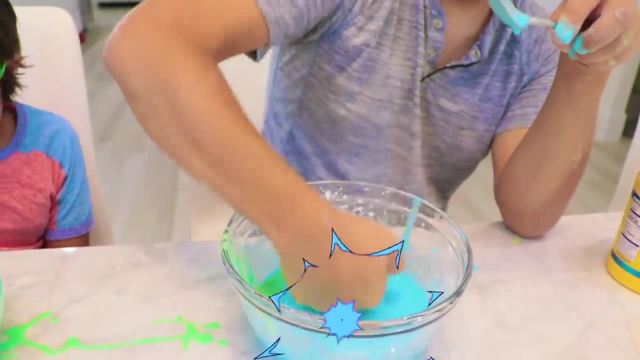 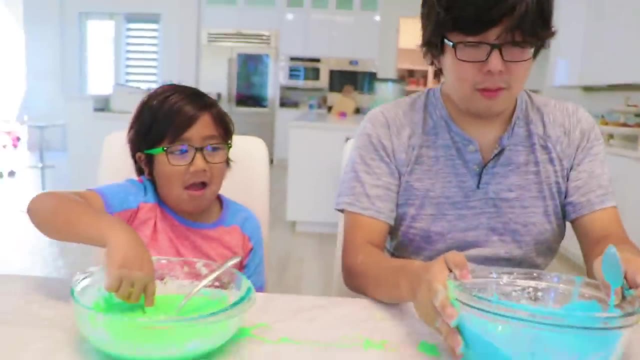 But yeah, I feel like it has both properties, Because this is like, look, it feels like solid, right, But then see It moves like liquid, Yeah, so I want you to pick up some, Okay, And put it and squeeze it between your hands. 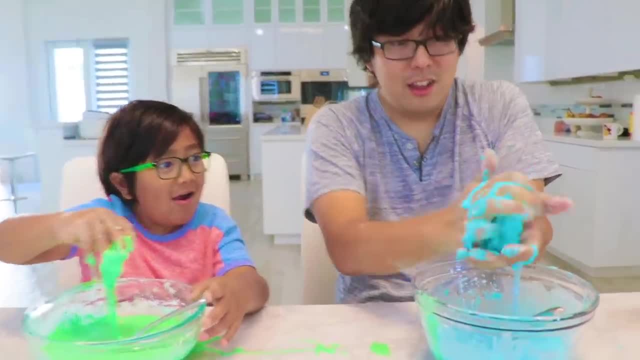 Does it feel hard or soft? It's hard. Yeah, when you put it in your hand it feels hard like a solid. I'm making a ball, right, Yeah, I'm making a ball. Let go, let go. So that's a solid. 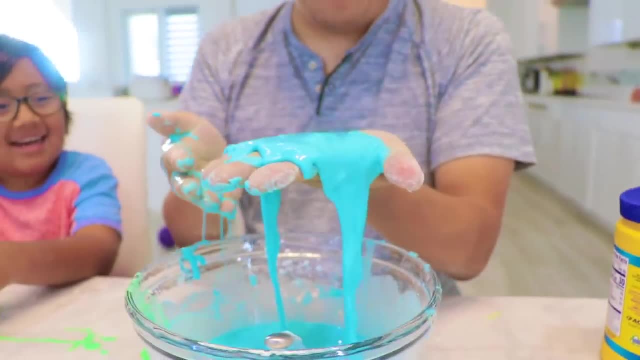 What happens when you let go? It's liquid. Yeah, I'm so confused. Which one is it? All right, you try, Ryan, It's both obviously Seven years old. it's teaching me. You try, You pick up a whole bunch. 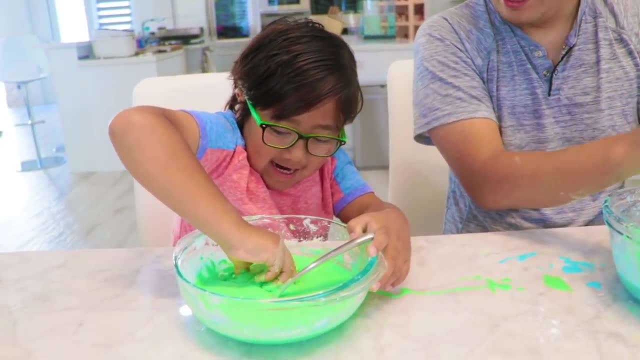 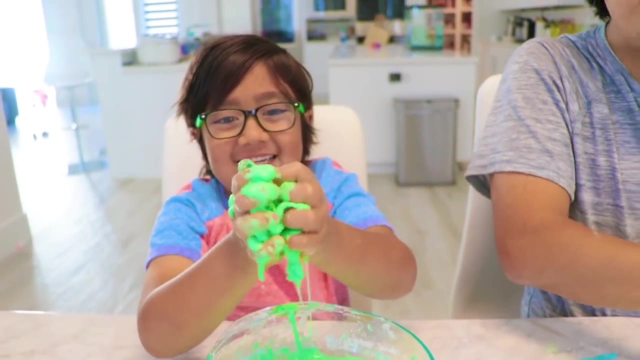 And then just squeeze it. Don't leave any space. Does it feel like a solid? Yeah, It's solid, It's solid, It's solid. Is it solid or liquid? It's solid, Yeah, but if you let go, what happens? 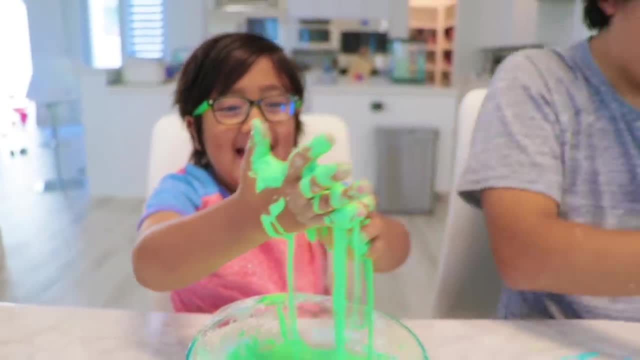 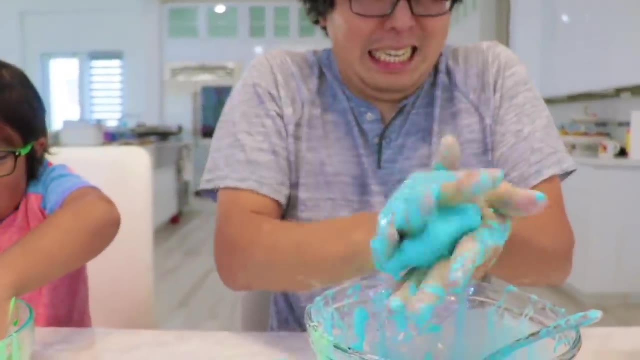 It becomes a liquid. Yeah, So it's not your typical solid liquid, right? So if I want to keep it solid, I have to do this forever. Yeah, It's melted. I'm getting mad, Yeah, so this is really cool. 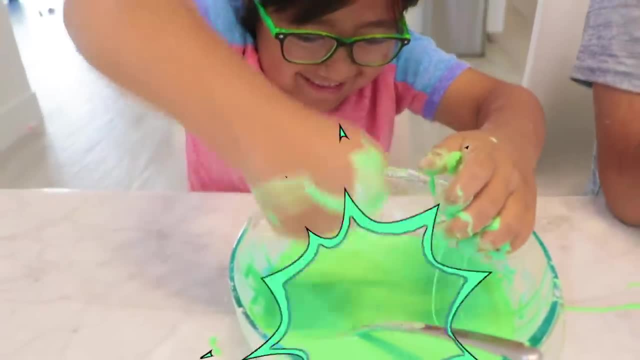 This is actually called a non-Newtonian liquid. Huh, Non-Newtonian liquid. Oh, I'm getting mad. Oh, I'm getting mad, I'm getting mad, I'm getting mad. It's called a Newtonian liquid. 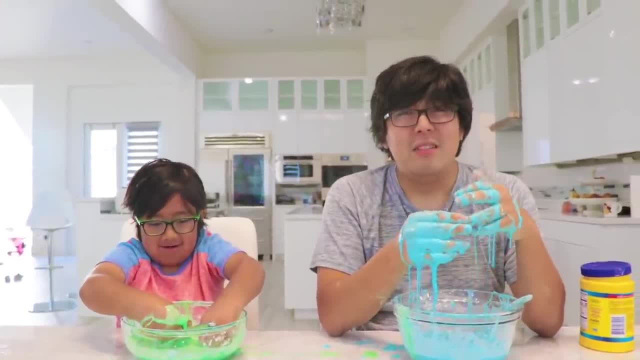 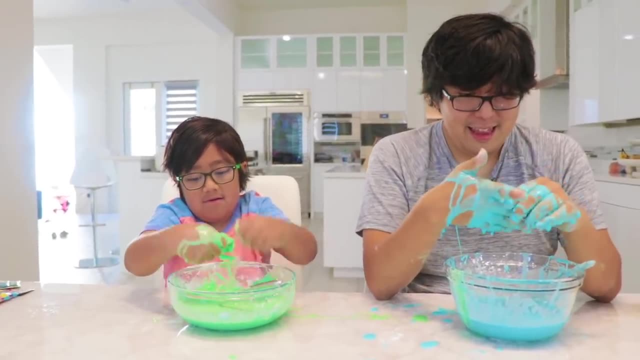 That's what it's called. What is Newtonian? Yeah, Newtonian after Isaac Newton. Okay, It's not a typical definition of a solid liquid and gas. It's a solid or liquid and it changes its property based on pressure. 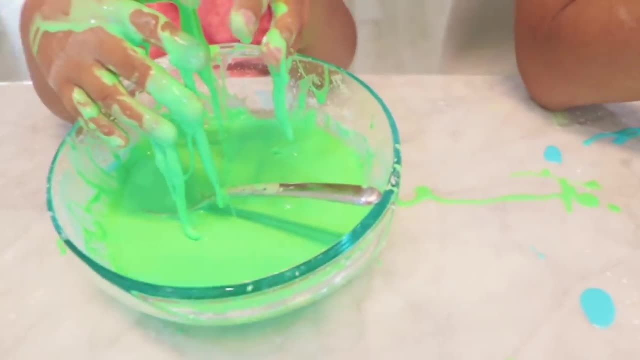 So if you apply pressure, it behaves differently. Mommy, you try to punch it. Okay, Mommy's going to try to punch. Let's see One, two, three. Whoa, That's super hard, like concrete. That's so fun. 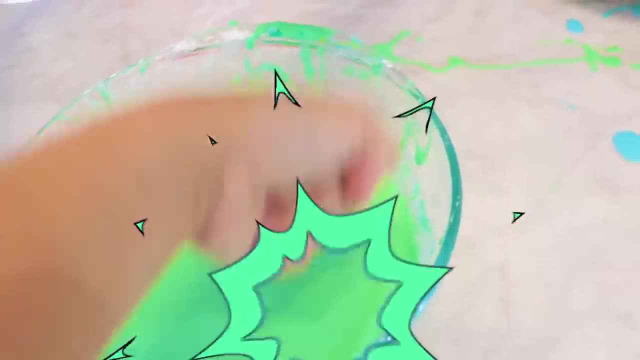 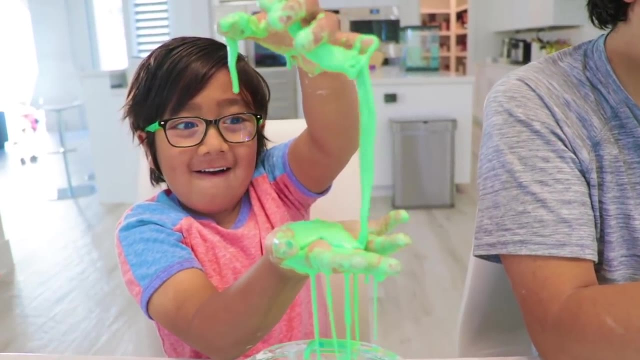 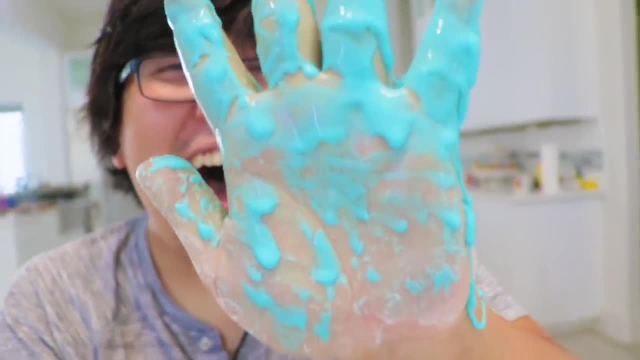 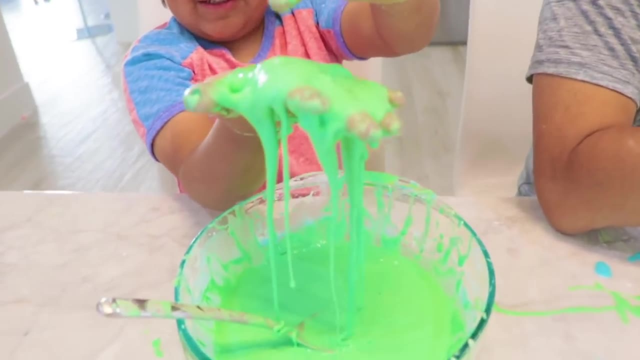 I'm melting, Wow Whoa. It looks like ice cream melting. Yeah, What flavor would that be? Matcha flavor? Maybe a Rocky Road? You can make your oob like even more exciting with adding glass. Wow, Which one. 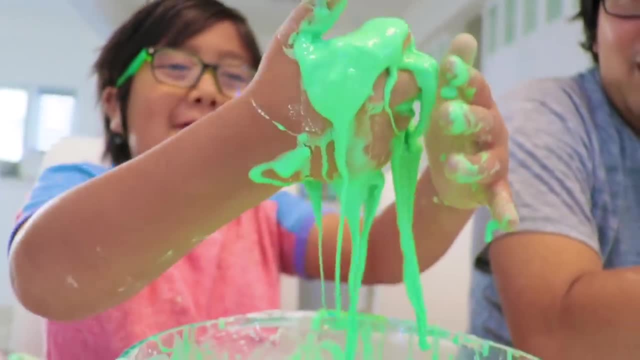 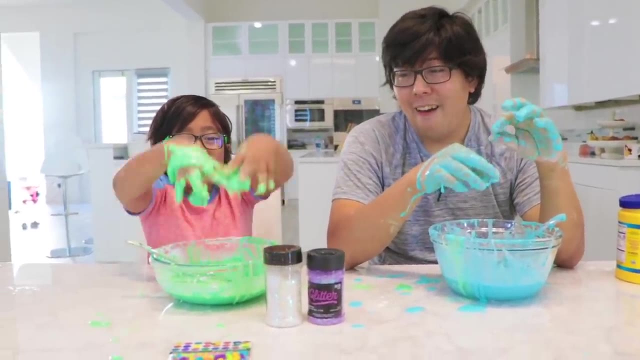 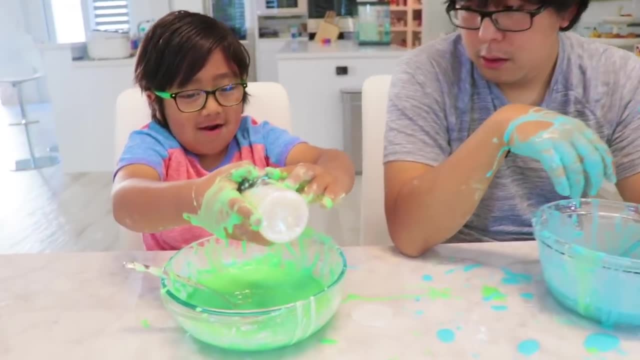 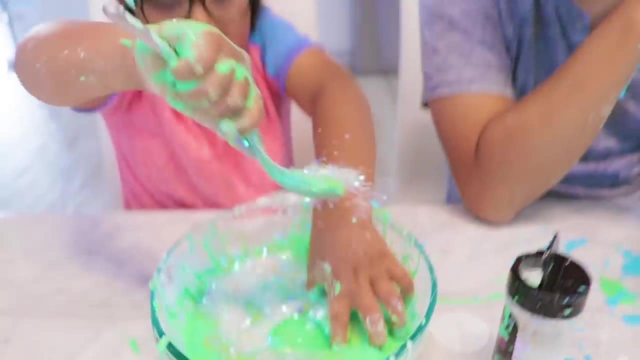 There are five. I want to do the bigger one. Okay, I get the purple one. Glitter- Oh, that was a lot. That's enough. Ryan, Shiny, Matt, How am I going to mix the glitter? It's on your hand now. 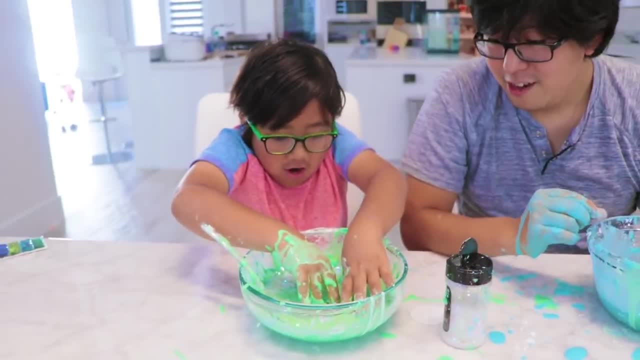 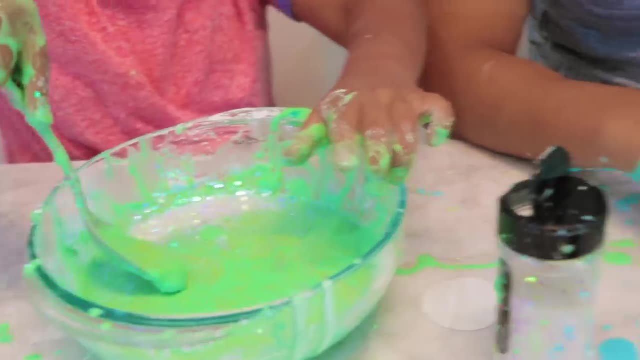 This is the only way I can mix it. Ryan added way too much glitter. All right, I'll do right. Oh, I need a lot more. I need a lot of glitter. Wow, Look at that, I like it. The only thing: it's hard to mix. 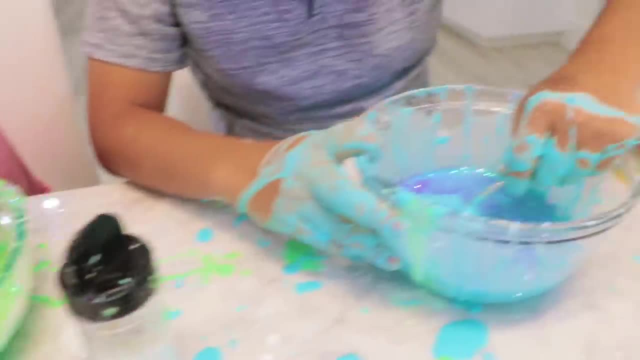 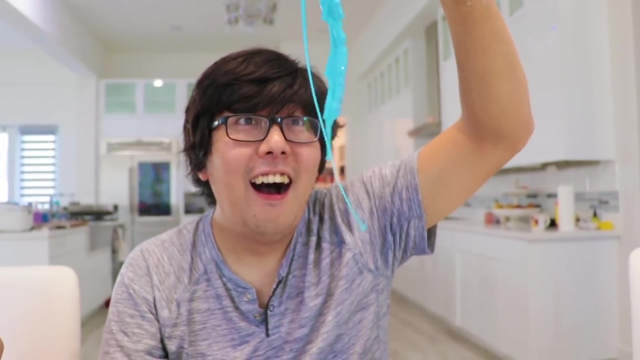 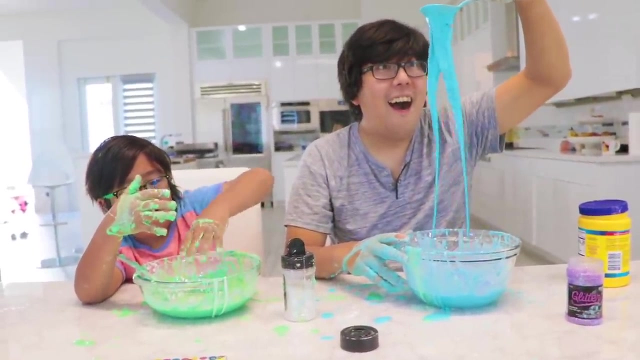 Do you see that? But if you leave it like this, it's actually hard to get out So cool. Okay, guys? so that's how you make oobleck, And when you're done playing, just do not throw it into the sink. 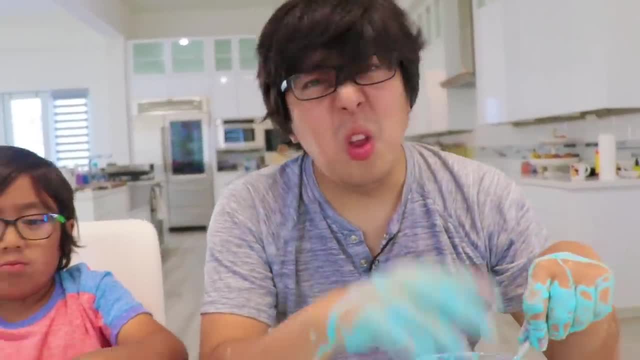 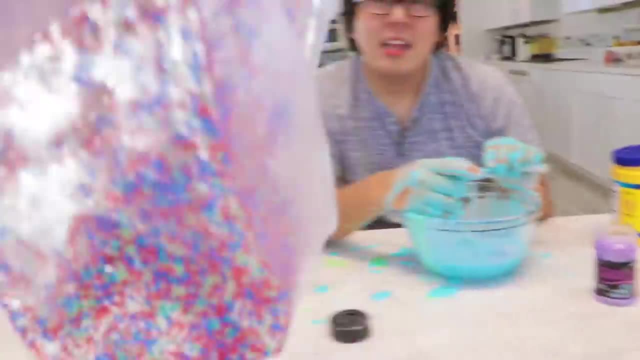 You know why? Why It could clog up your sink. Oh no, no, no, no, no, I don't want that. So if you're done playing, you just throw it in the trash, Or you can just put it in a Ziploc bag like this: 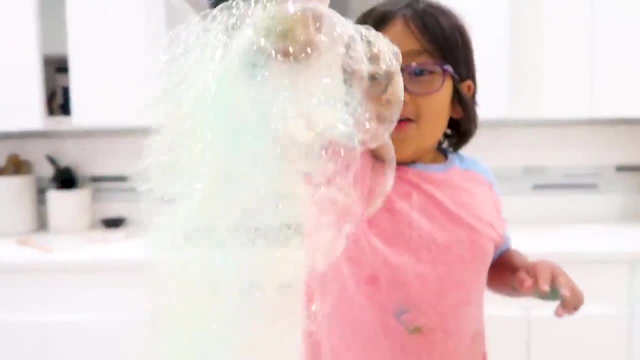 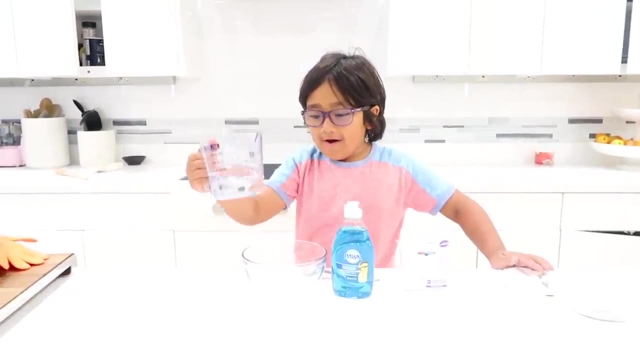 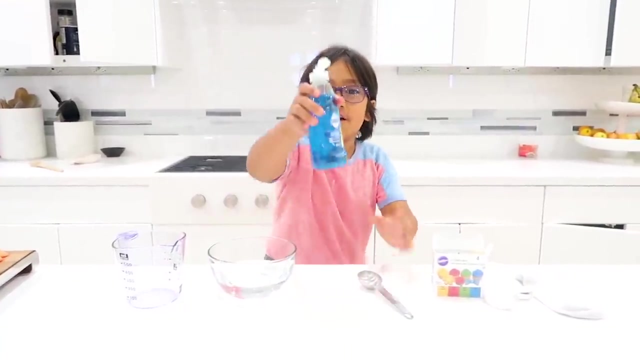 So you can play again later. Next is how to make your own bubbles at home. Hi guys, Today we're making colorful bubbles. So you get water and you put it in About one cup of water And you need two tablespoons of dog soap. 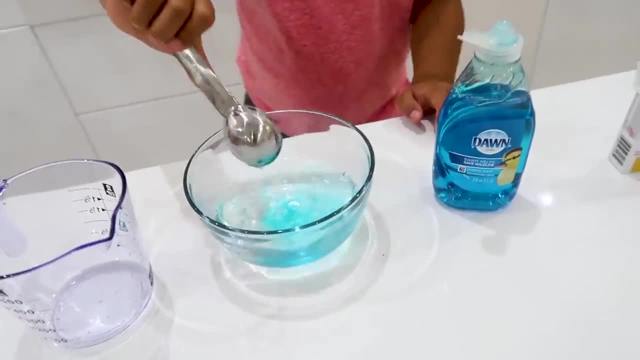 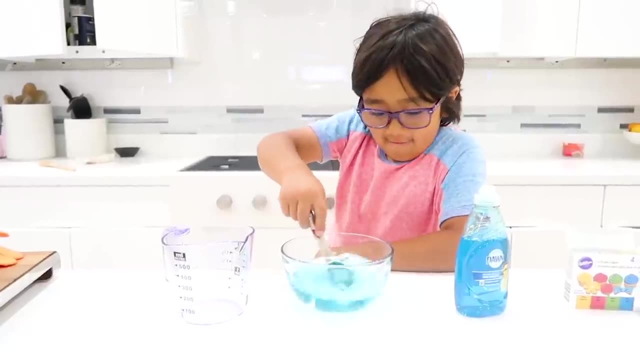 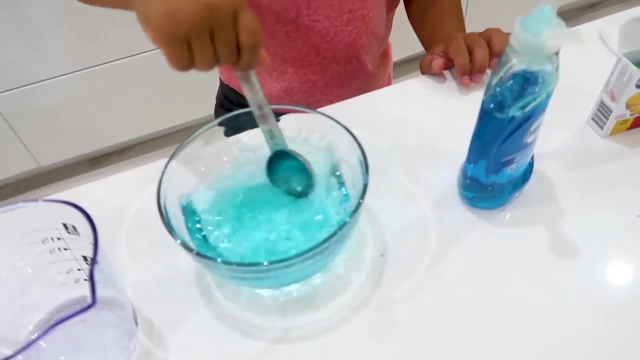 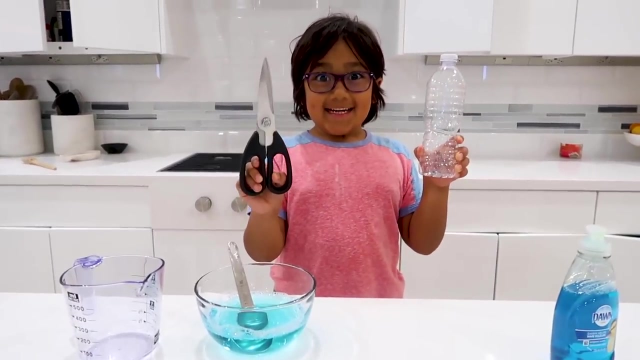 One, Okay, Two. So next you're going to just agitate and mix it together. One, Two. Next you're going to need a bottle And ask a grown-up to cut it for you like this. So I'm cutting it for Ryan here. 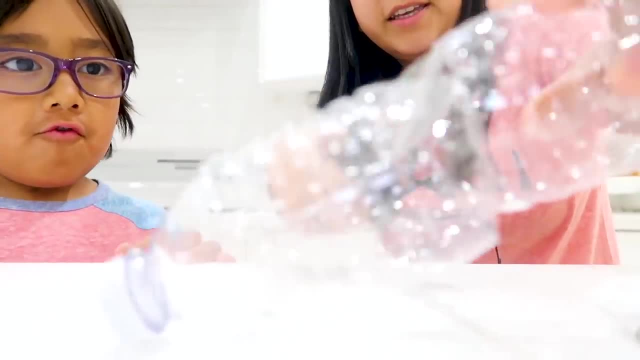 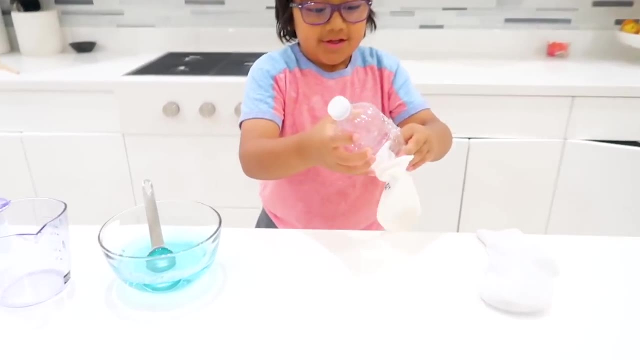 So like this, It doesn't have to be perfect. There we go, Cut. Next you're going to need a sock, And then you're going to put the cup inside. So now I'm going to help Ryan with it. So there it is. 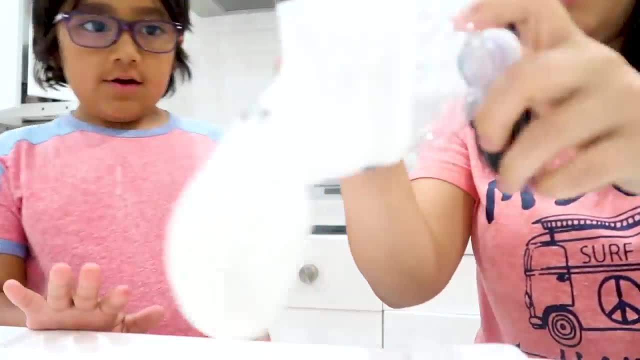 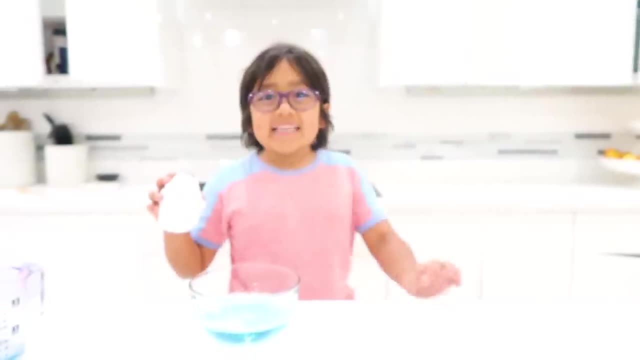 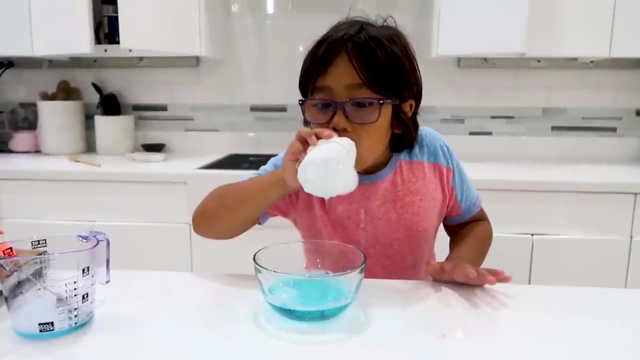 You just put it in like this. It looks something like this: Next you dip it in and then you blow. There you go. Now you're going to blow out and not in. Okay, So you see what happens there. Look, Whoa. 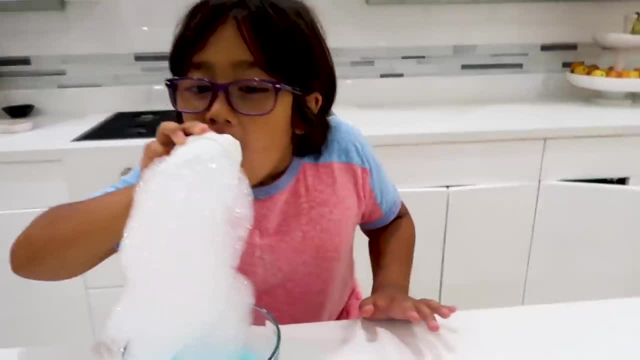 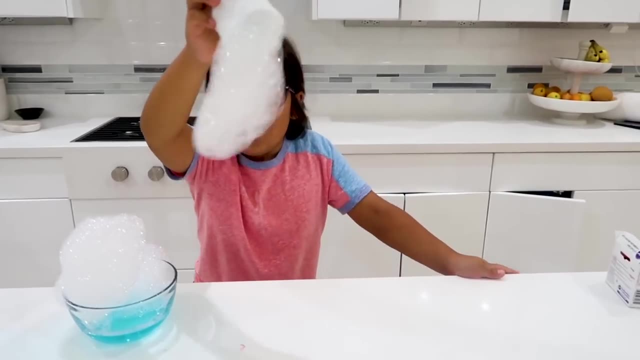 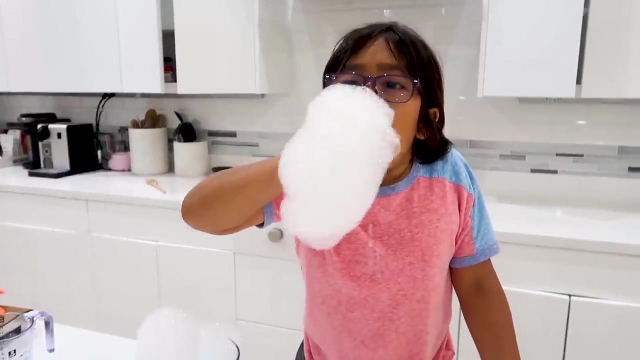 Let's see how long Ryan can make it. Oh, it's going into. It's going into the solution, Ryan? Oh, All right, Keep blowing and see how long you can do. Look, Don't forget, you have to blow out and not in. 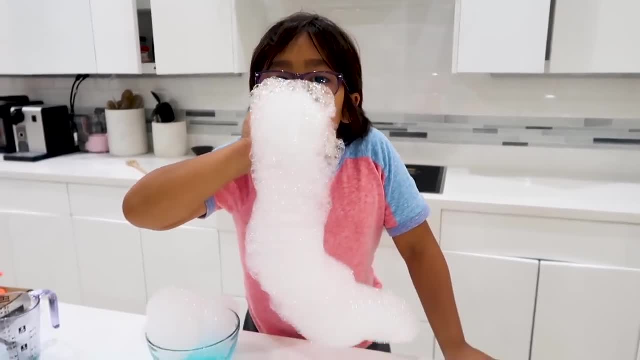 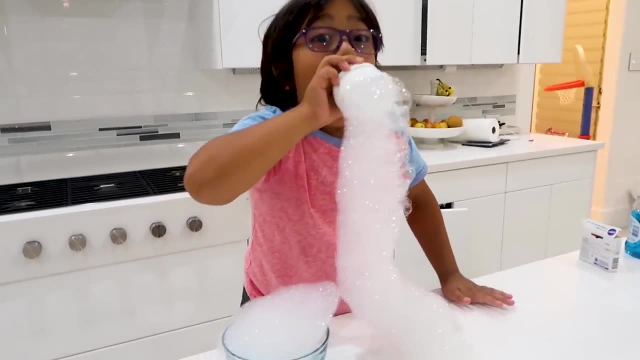 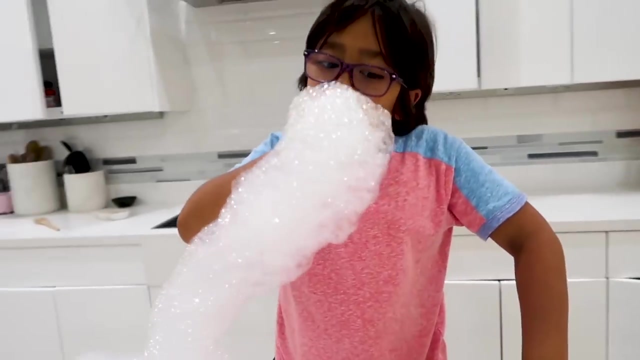 And this is best for, maybe, kids over five years old. Make sure you do this. Make sure you do this. It's a parent. Look how long Ryan is doing it. Whoa, Super long. You guys see how long he did it for. 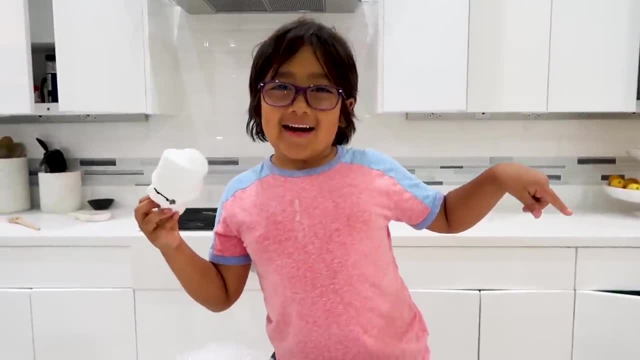 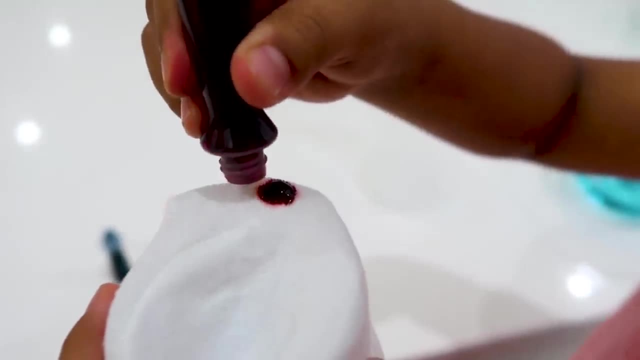 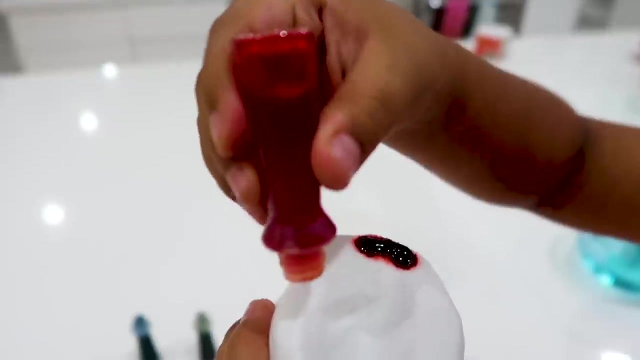 Whoa. Now let's add some color. Now we're going to add food coloring. This is red. I'm going to put a few more drops. This is yellow or orange. Yeah, I think the ones drop, Drop, Drop. 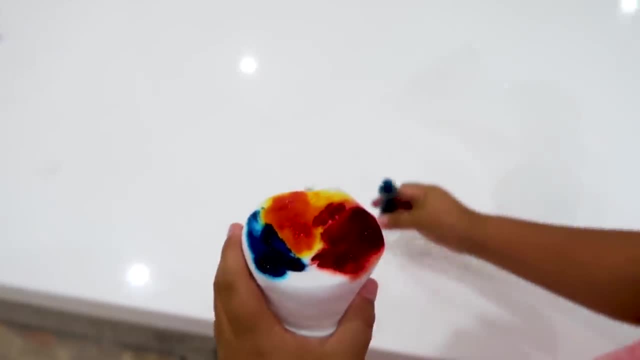 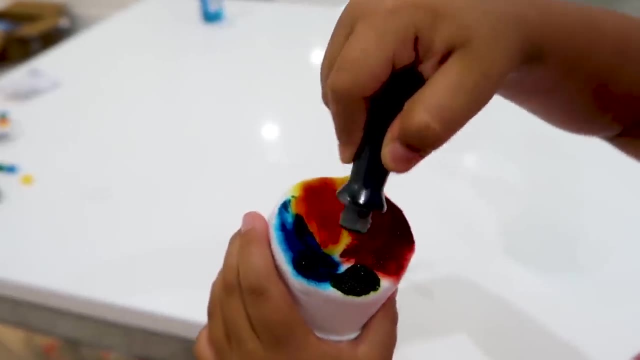 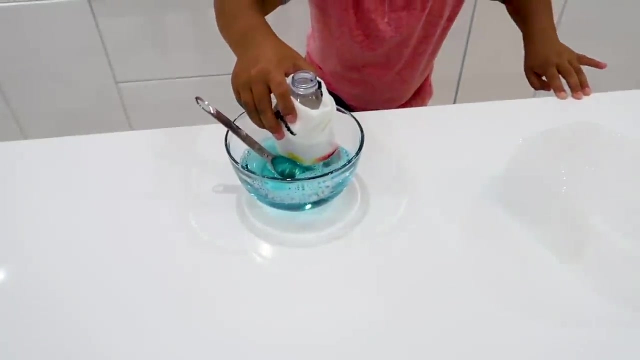 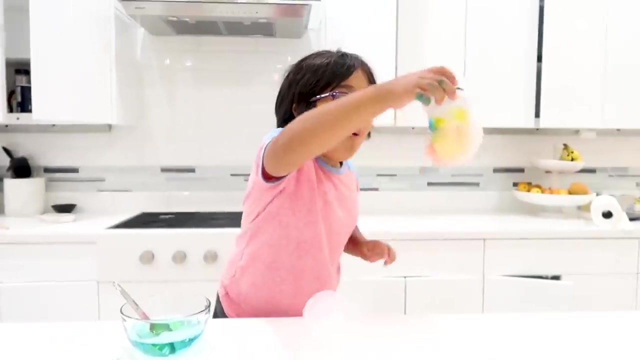 Okay, Now we're going to do blue. Whoa, Now we're going to do green. Now we're going to put it in Dawn's soap In water, In water, In water, Ooh Whoa, We mixed the colors. 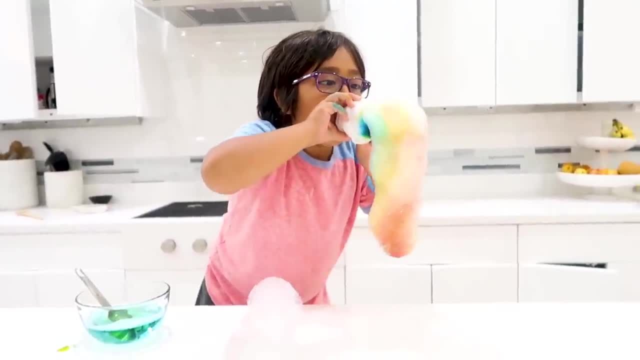 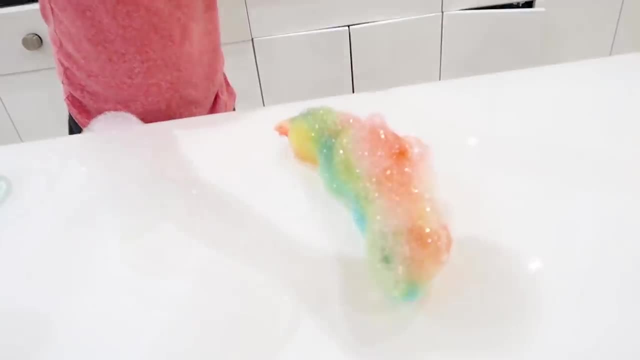 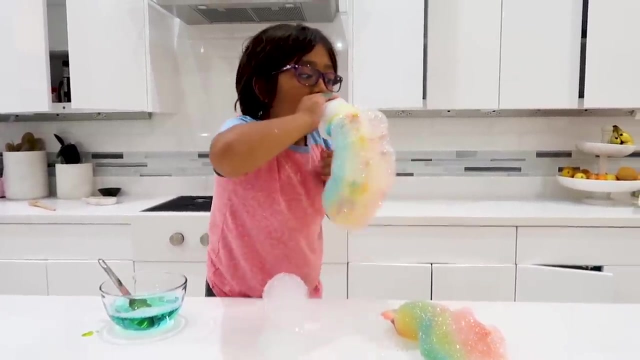 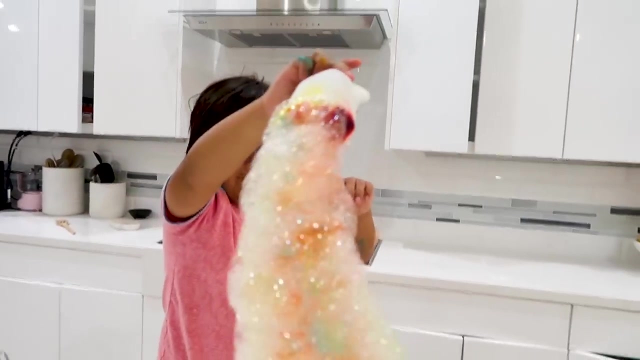 Whoa, Look at this bed. Remember to blow out and not in. Whoa Lo ON. Haha Hi, Why have you been up all night? W Alego, Are those good? that looks cool. okay, guys, I actually made my own too, so we're gonna do it together. 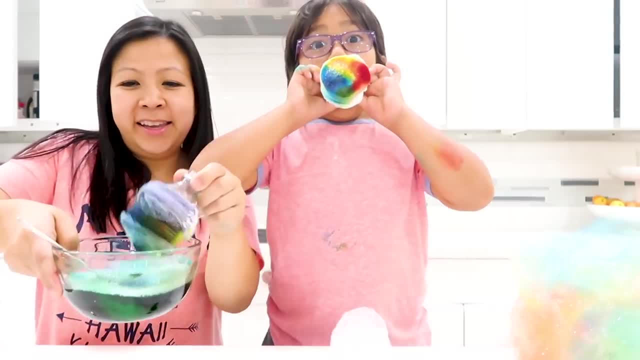 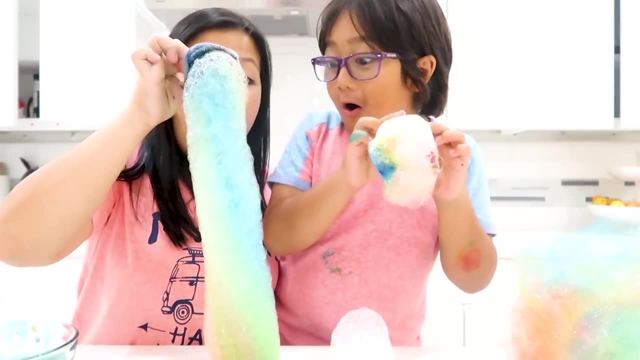 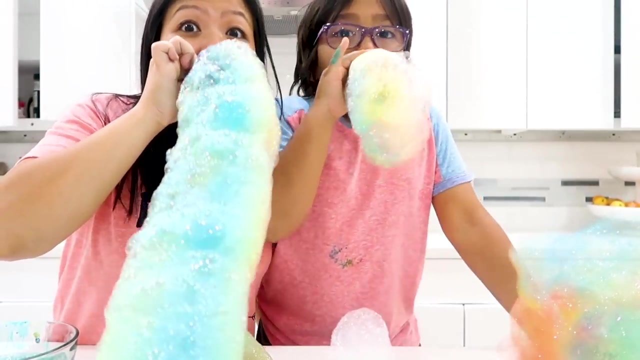 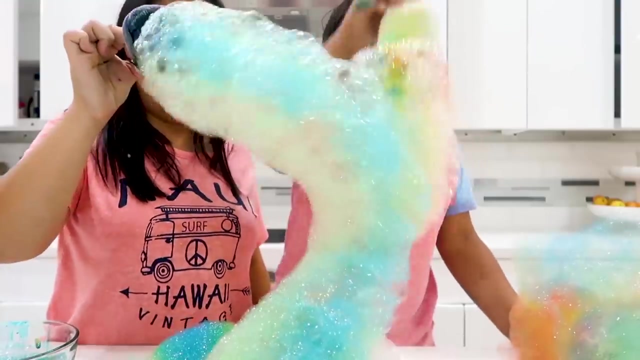 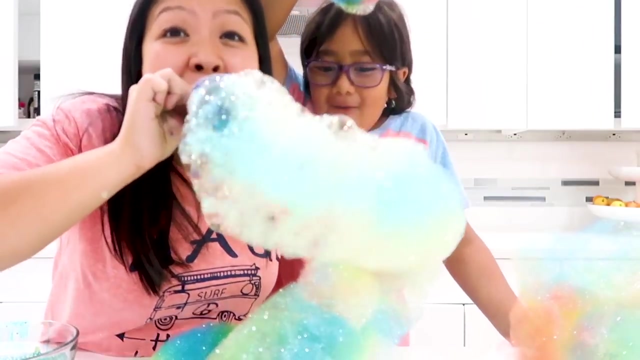 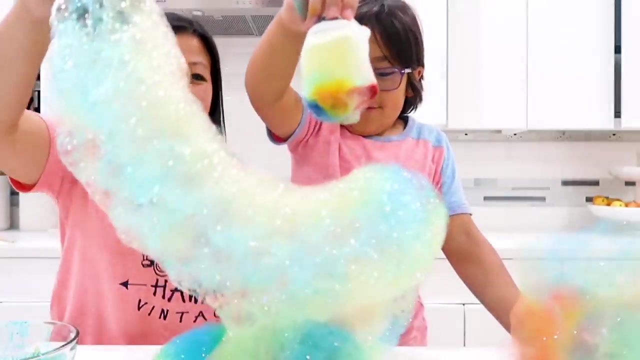 okay, all right, I'm gonna dip it in. okay, you ready, Ryan? one, two, three. wow, how can you do it so long? so I guess I'm meager, so I can make more. look at this: Whoa, maybe mine's better. I could try mine. 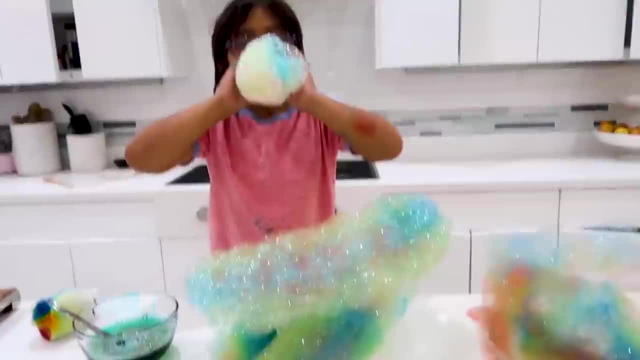 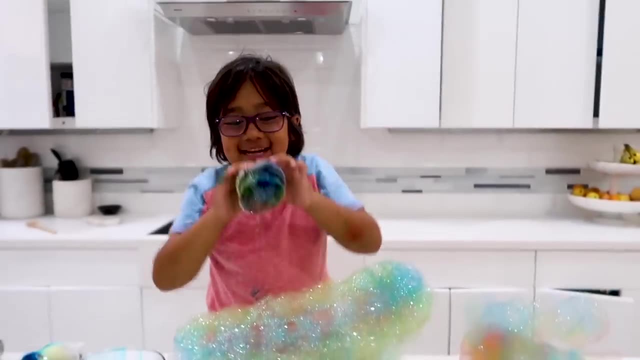 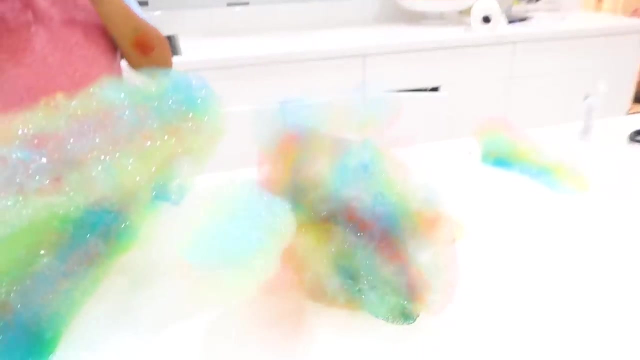 Okay, I guess if that was my pile over there, Ryan's gonna just what? do you think Is it any better? Whoa, Ah, It's so warm. Do you think it's any better? Oh yeah, Whoa, that's fun. 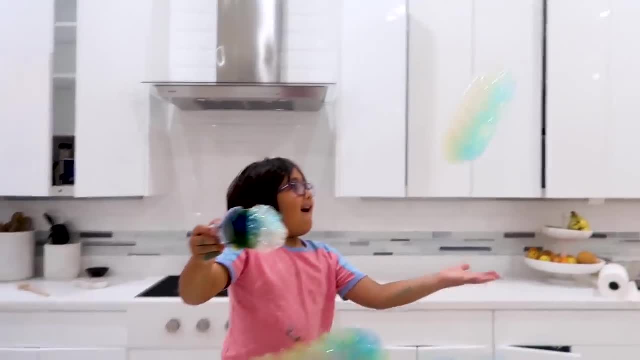 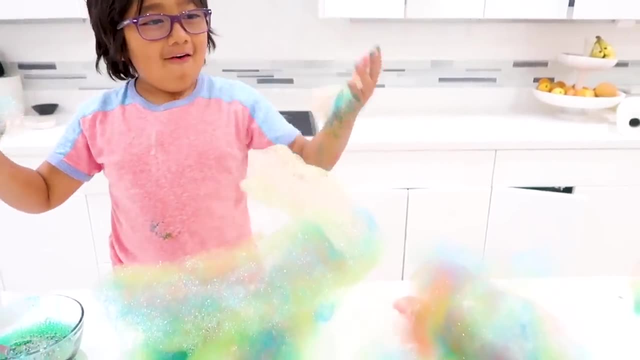 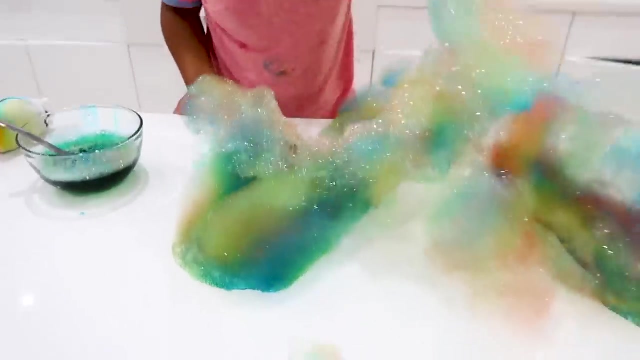 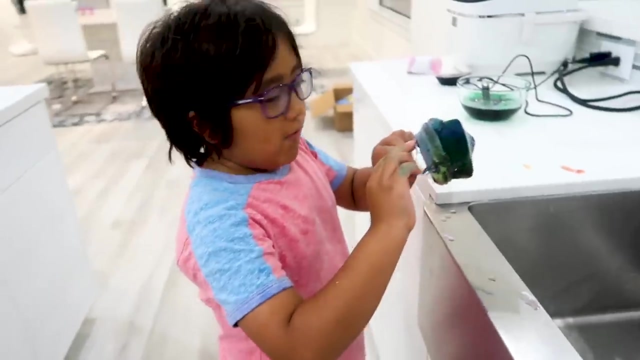 Whoa, Whoa, Whoa, Whoa, look, look, look, look, look. I know. Okay, guys. so now we're doing the challenge of doing it in our sink. Ryan's gonna do it, I'm gonna do it too, all right. 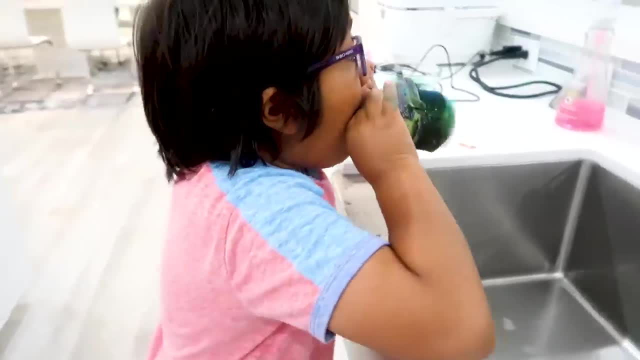 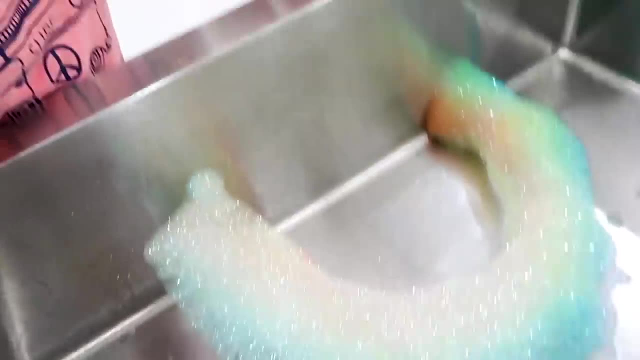 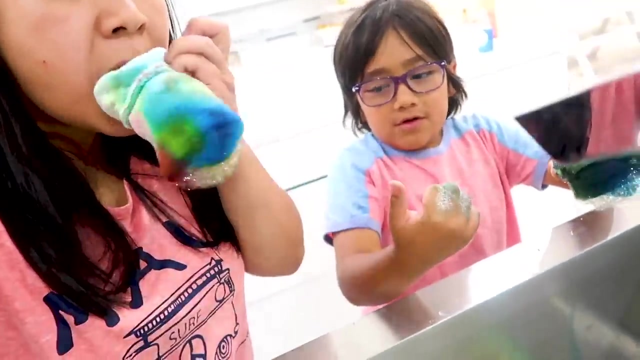 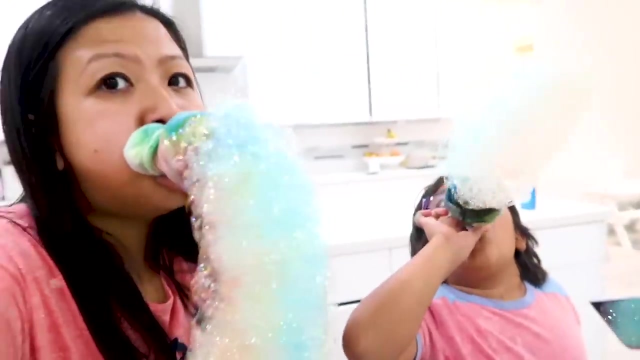 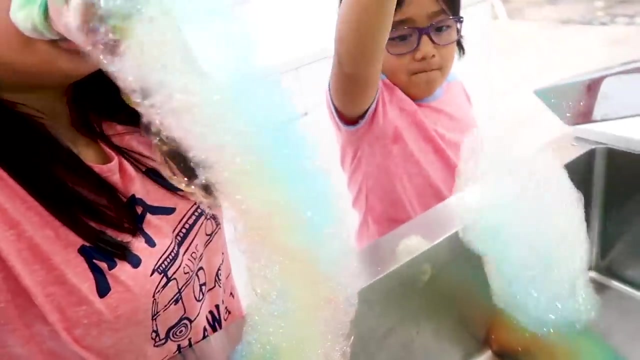 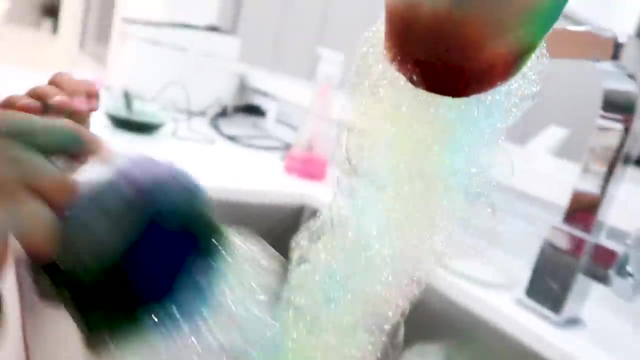 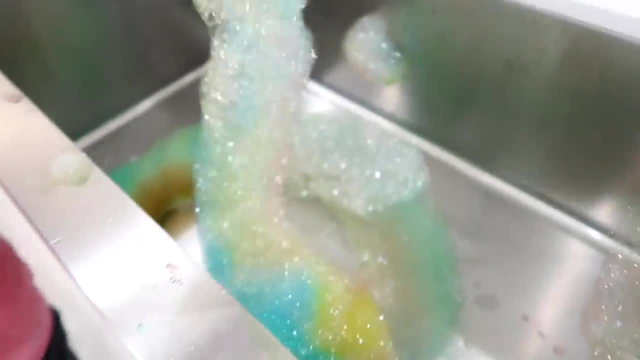 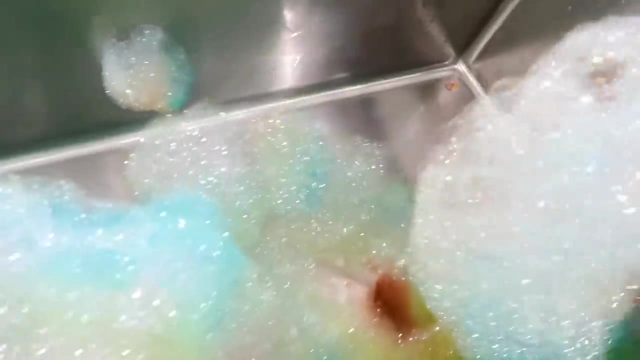 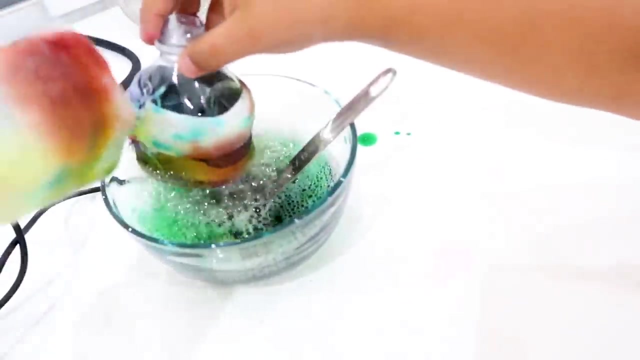 Hey, bubble fight, Whoa Whee. Okay, guys, this is how much we got here in our sink. It's a lot Having fun, Ryan. Yeah, All right, we're gonna do one more flow for you guys. 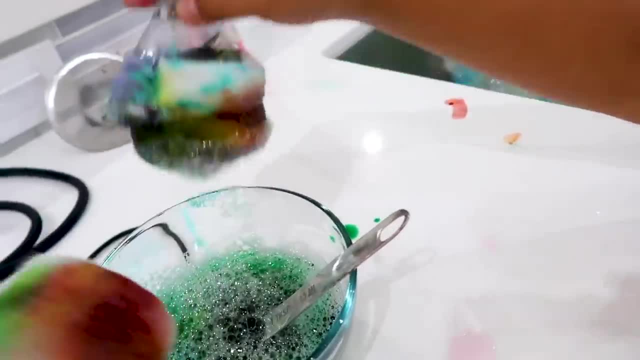 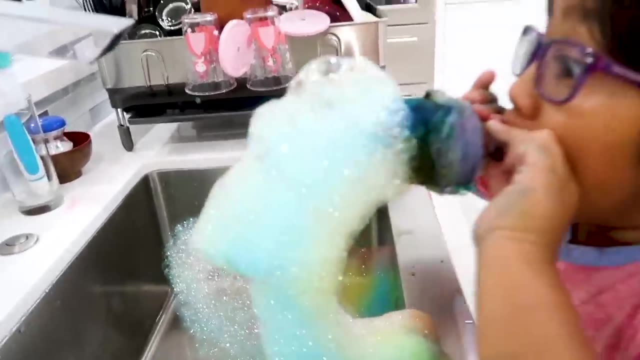 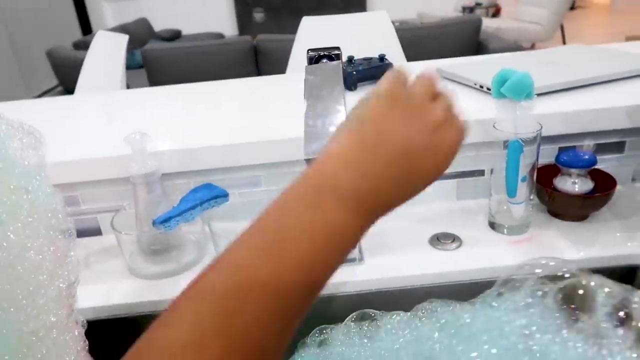 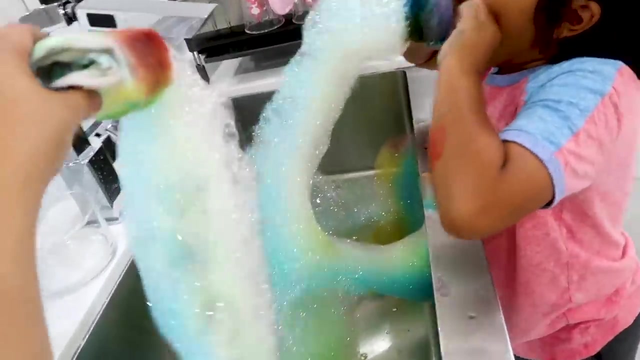 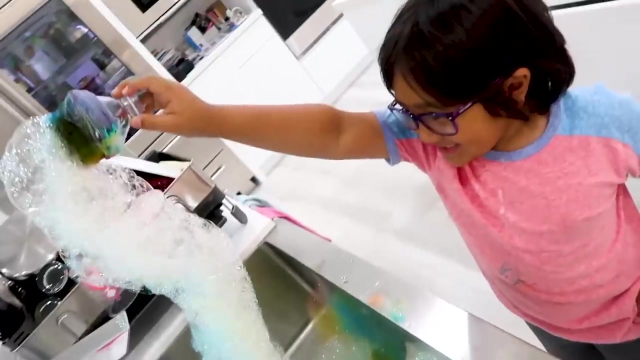 The in-sink radiator can't stop us. All right, One, two, Woo Whee. Bubbles, Ah, Whoa, Oh, ba-ba-ba-ba-ba-ba-ba Bubbles whee. 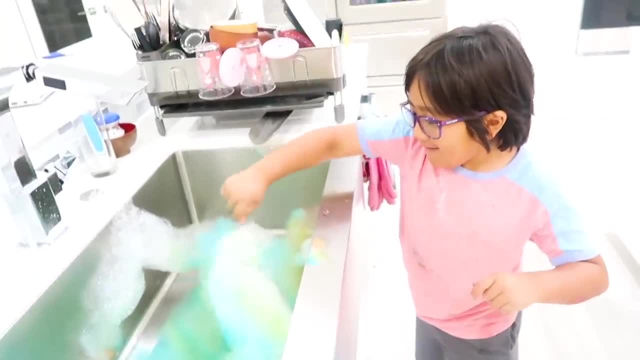 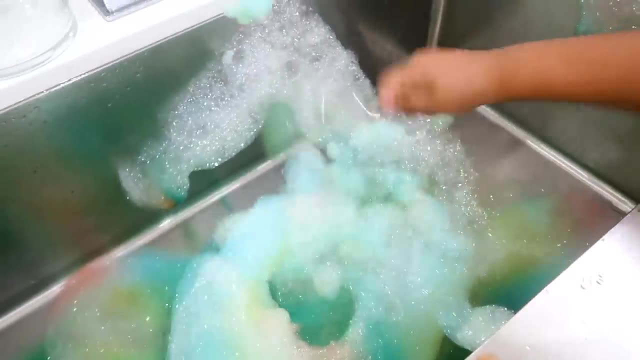 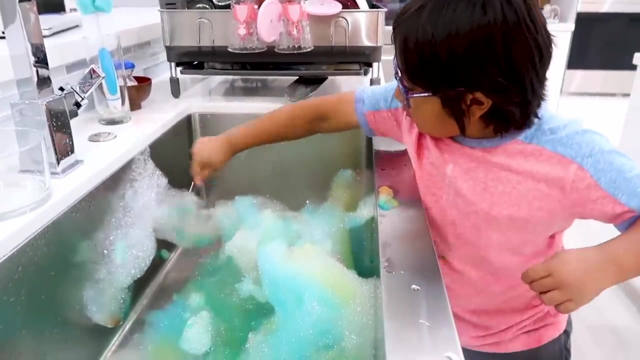 Bubble fight. yeah, yeah, yeah, Ba-ba-ba-ba-ba. Ryan's having a bubble fight. I'm fighting the bubbles. Who's winning? Ryan or the bubbles Cut? This is easy way to make your stick figure float. 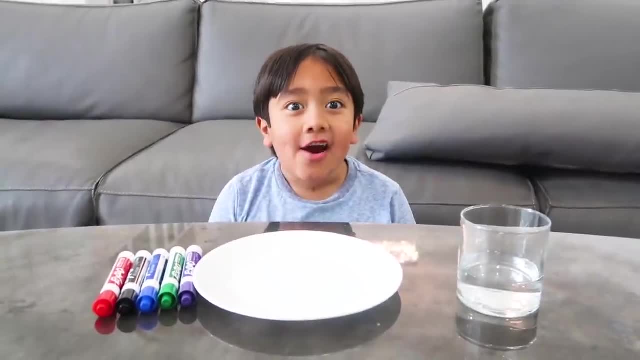 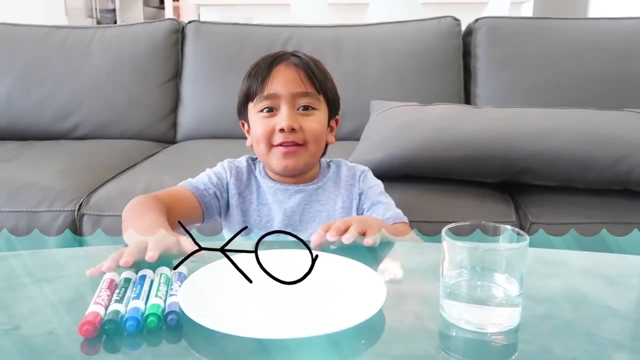 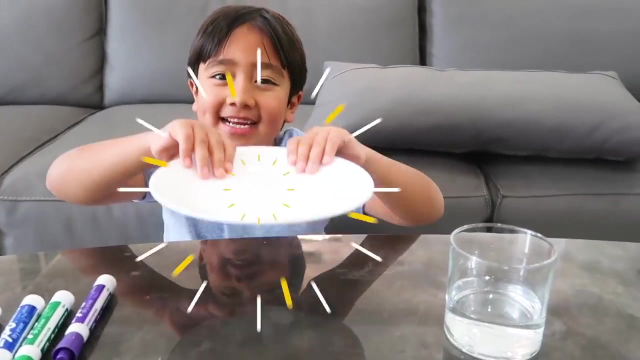 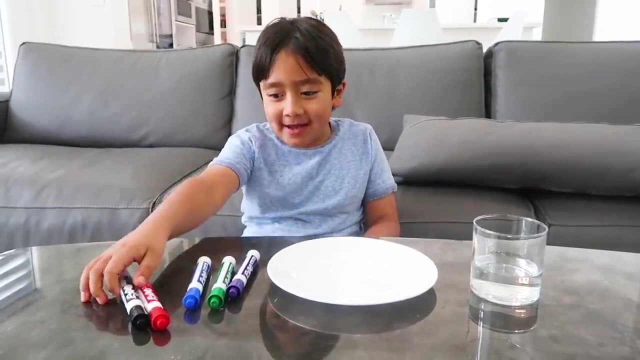 Floating marker trick. Hi guys, Today we're gonna put our trawling and then make it float on water. So this is very easy. All you need are some markers, a plate and some warm water. First, draw what you want on the plate. 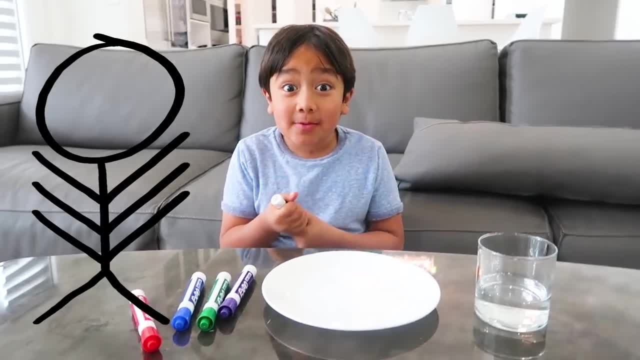 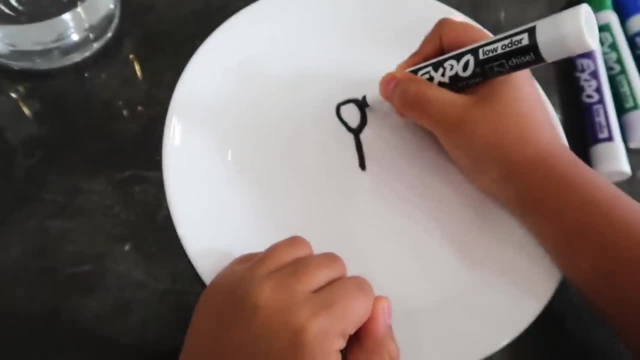 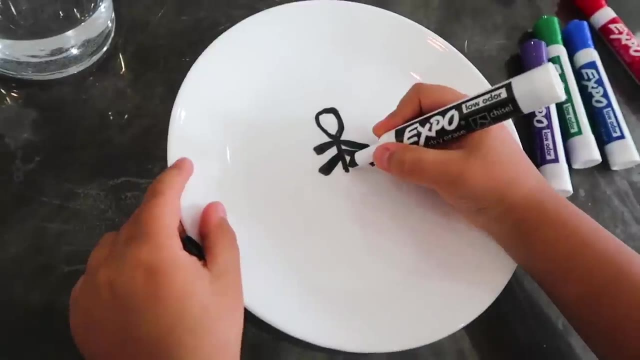 Well, I'm gonna make a stick figure with multiple arms, What? So? I'm gonna make it like this, And then you make it really thick, Like this, And you make arms, And then you make the legs. So, after you make your trawling, 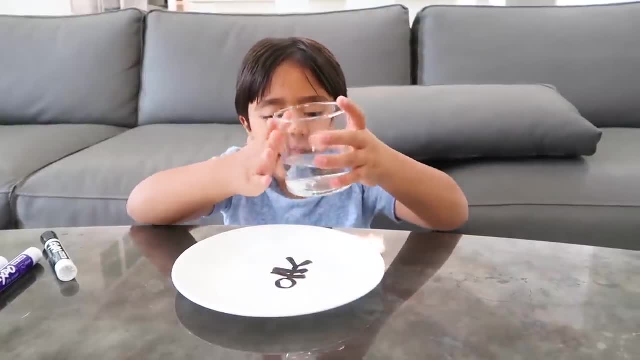 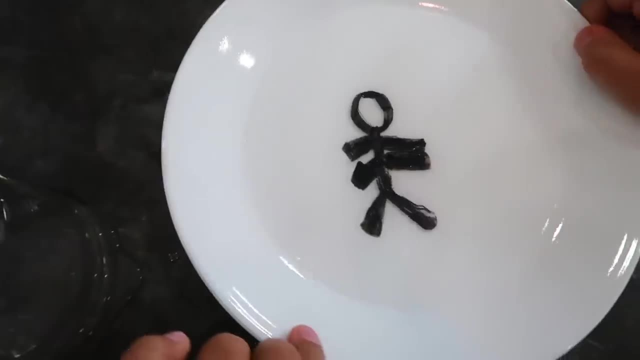 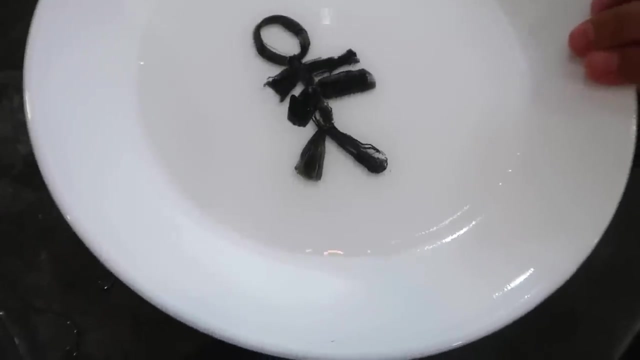 then you put some warm water on this side. Whoa, he moved. Look he's dancing. Ooh, his arms too. Ah, I feel like the arms or legs are gonna break. Oh, it's moving now Yay. 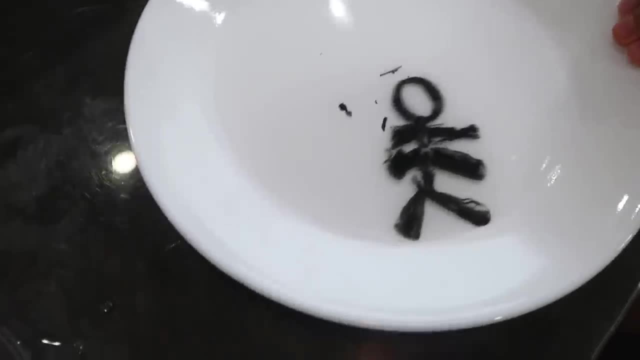 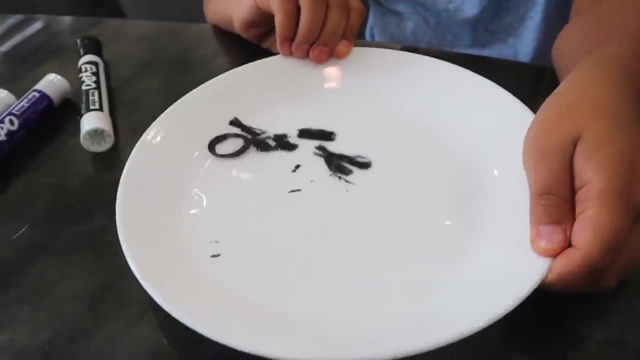 Now he can just walk. Do, do, do, do, do do. There you go. This is easy way to make your stick figure float. Do, do, do, do, do do. Oh, He broke. This is so cool. 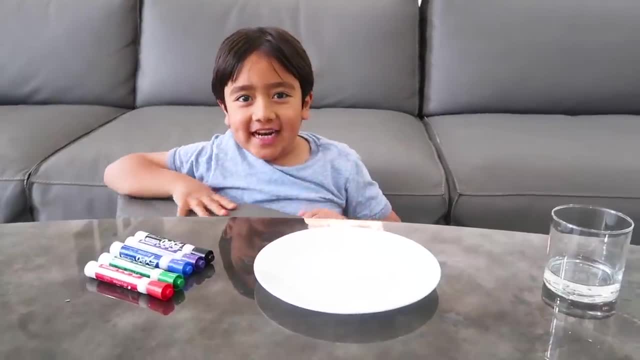 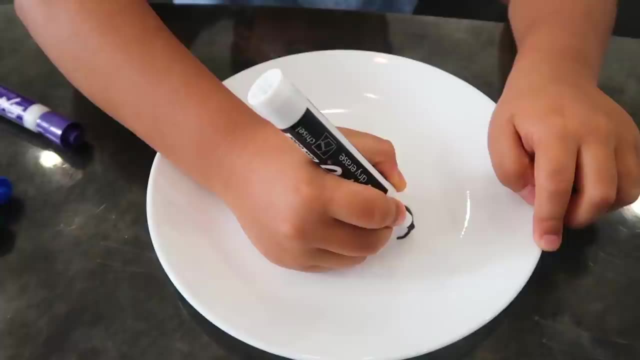 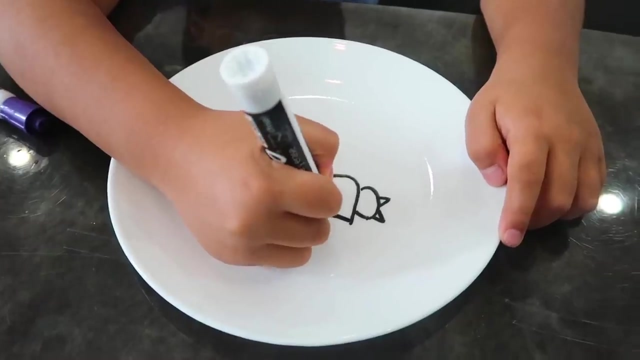 You can hold it. Okay, guys, On the next one, I'm gonna make a dog. It should be like this, And then maybe I can put like ears. I feel like I'm making a cat. I'm making a big dog or cat. 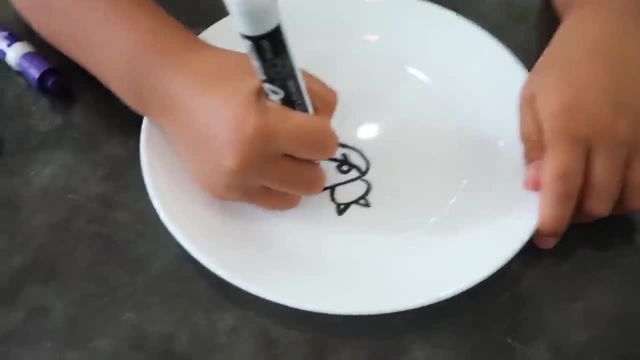 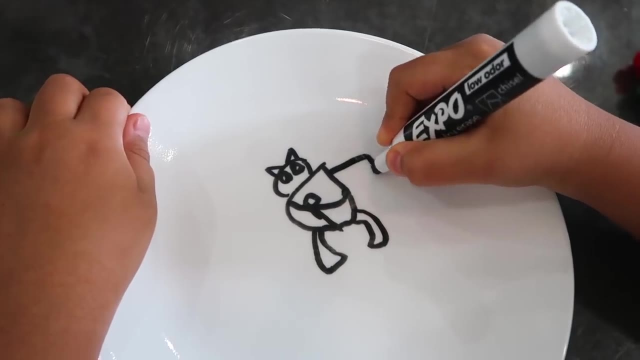 Oh, I can't do it right, Unless I do like this, I put an R. Okay, then I'll make the legs And then the arms. I feel like I'm making like a super strong cat or something. 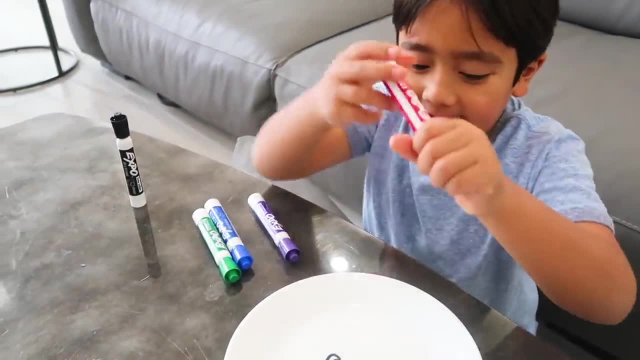 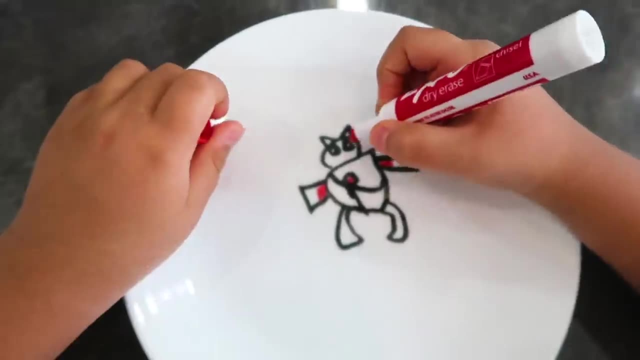 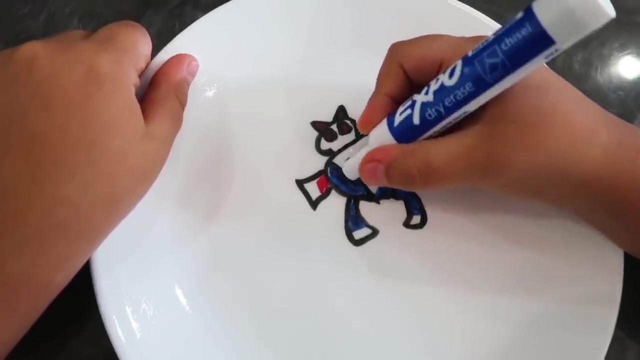 Meow. Okay, now I'm going to put a red right here And then I'm gonna make this red, And then I'll make the eyes red On the ears. Okay, so I'm coloring the pants. He has jeans. 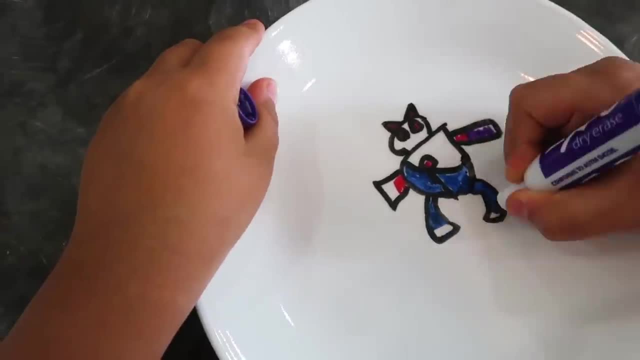 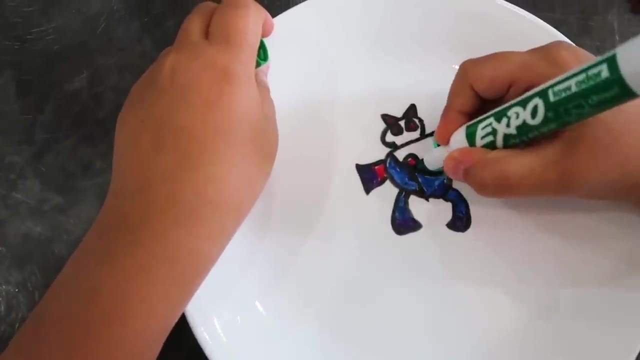 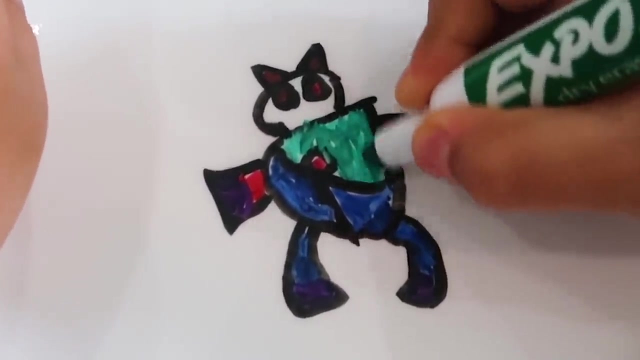 Okay, I'm gonna make the skin color purple. Okay, I'm gonna put it here And I'm gonna put this here, Okay, And I'm gonna put this part green. Okay, like this And Perfect. Okay, guys, let's see if it floats.